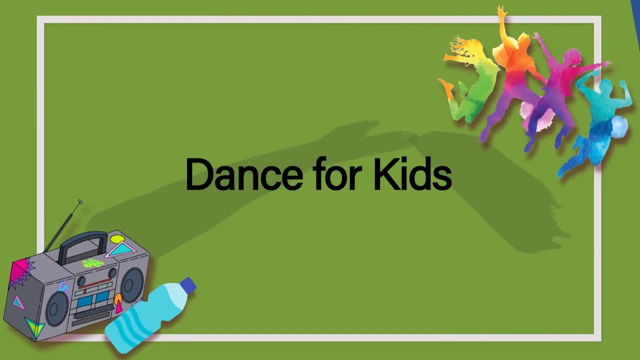 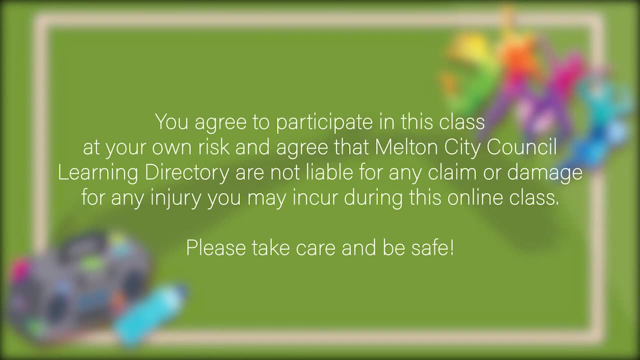 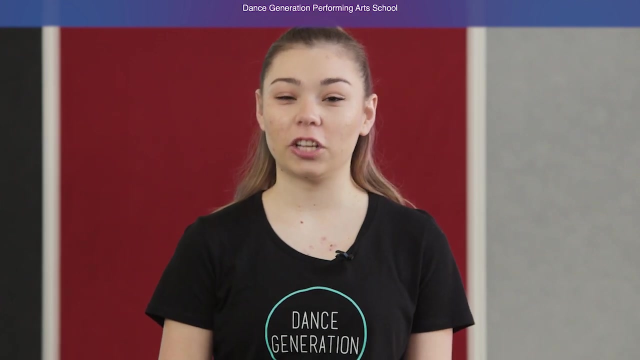 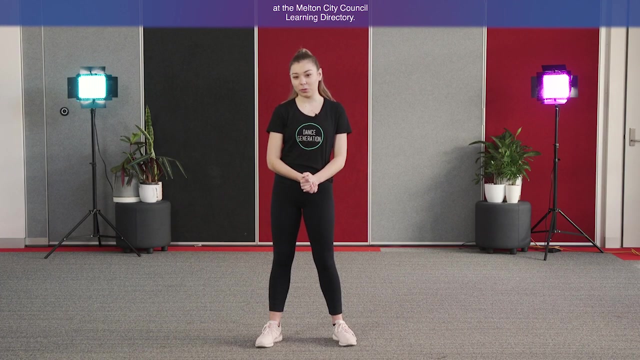 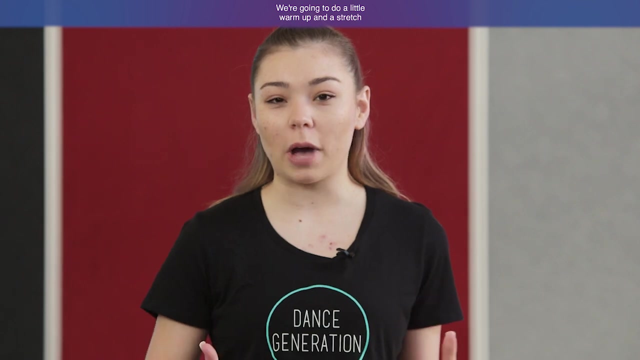 Hi everyone. I'm Ebony and I'm here from Dance Generation Performing Arts School And today I am dancing here at the Melton City Council Learning Directory. And today I'm going to be teaching you a jazz routine. We're going to do a little warm-up and a stretch and then we're going to do a dance. 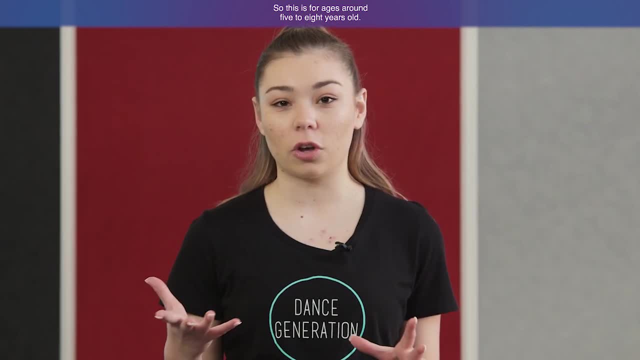 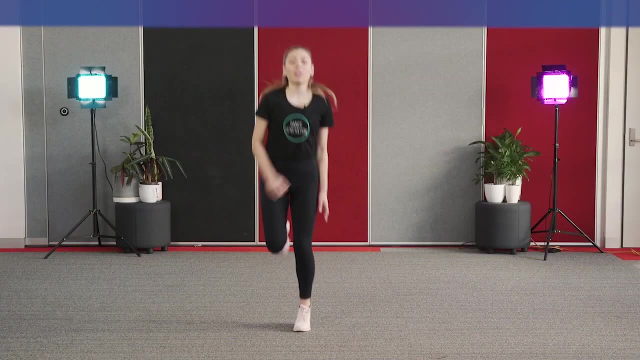 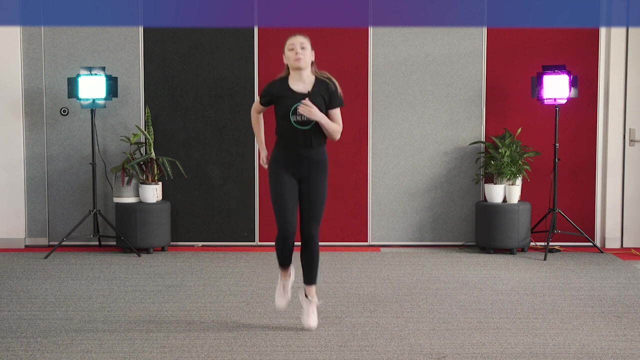 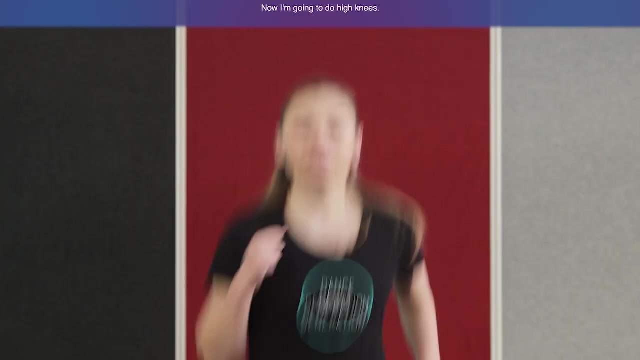 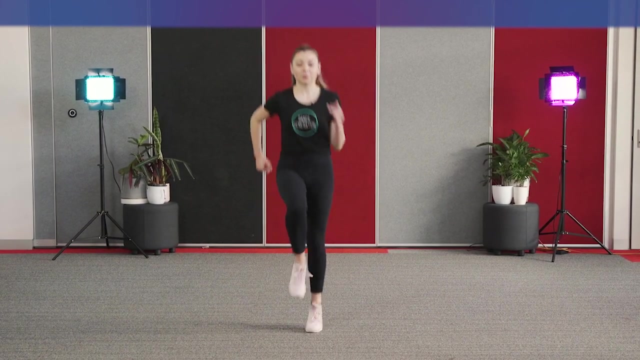 So this is for ages around 5 to 8 years old. It's a little bit challenging, but just give it a go and have some fun today. So we're just going to start off with a jog in time with the music. Now we're going to do high knees. 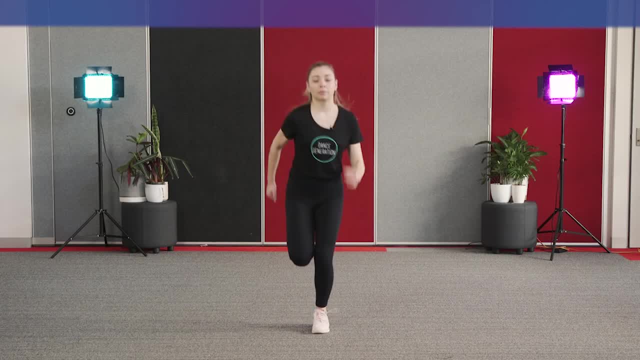 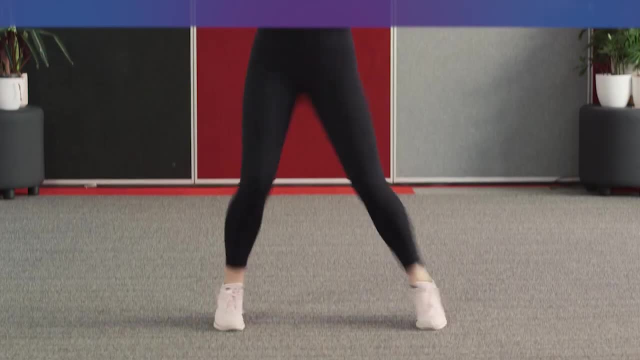 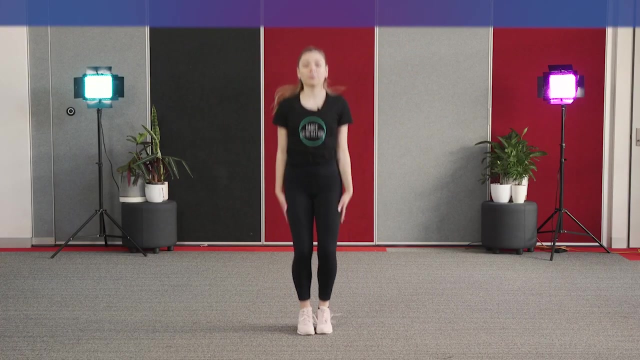 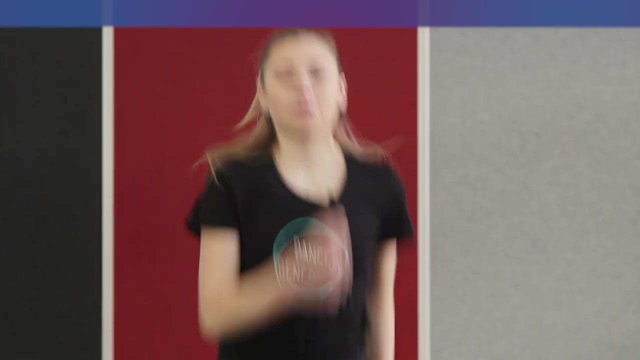 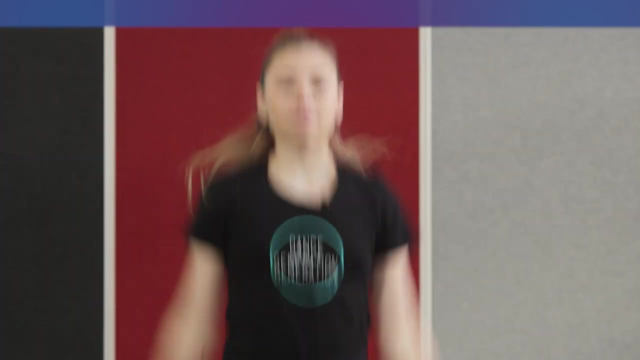 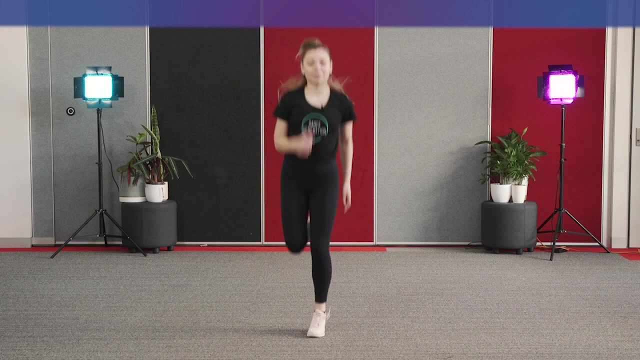 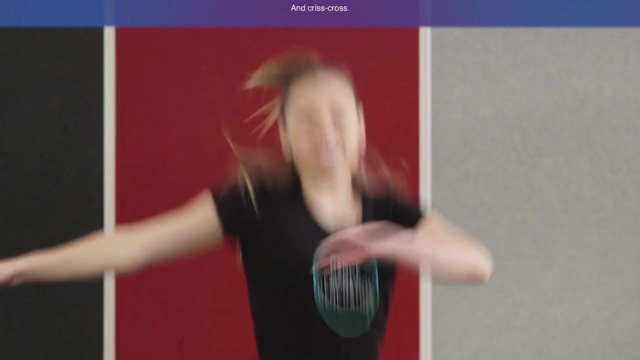 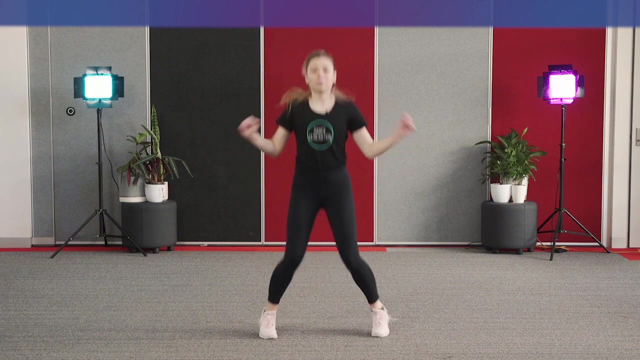 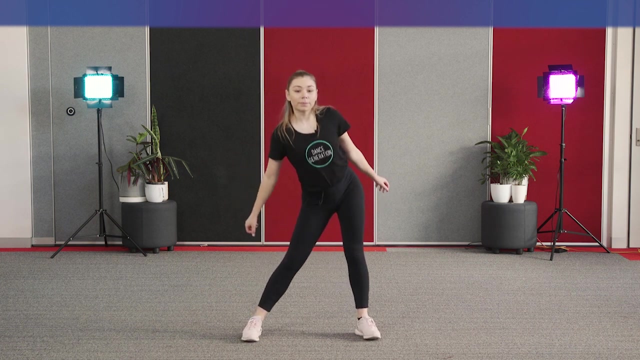 And back turning again And side jumps And double And running again And side jumps And number 4.. And side jumps And pull them back, twist and criss-cross. good, really big hips. Now we're going to do really big circles of our hips round. we go other way. 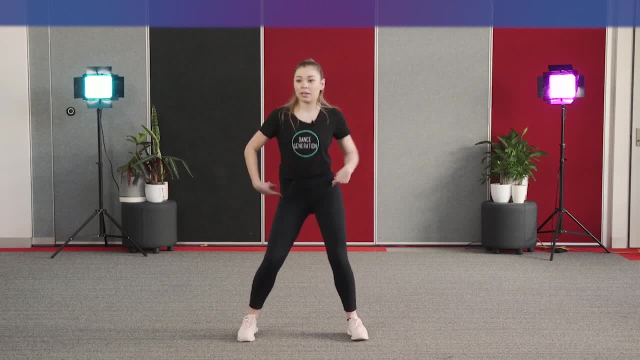 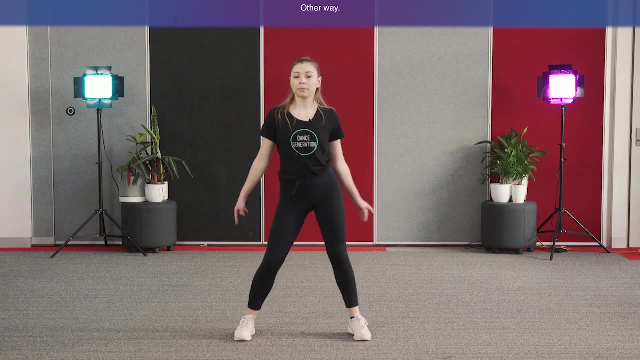 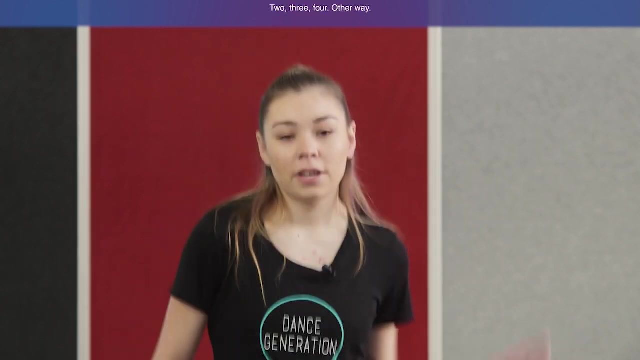 And now we're going to do really little ones. so really use that hip Good. And now we're going to do really big circles of our hips round. we go other way And for four, two, three, four- other way. 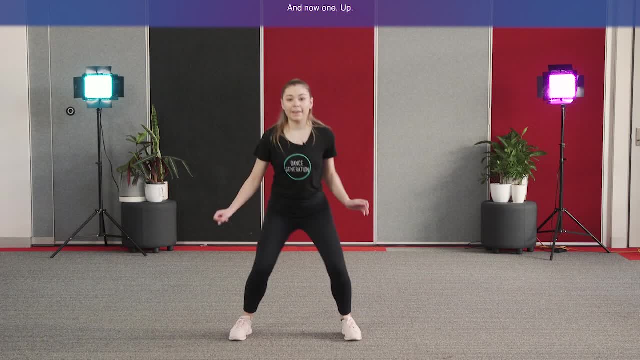 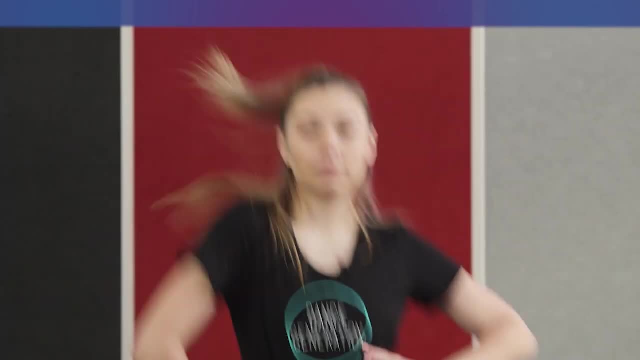 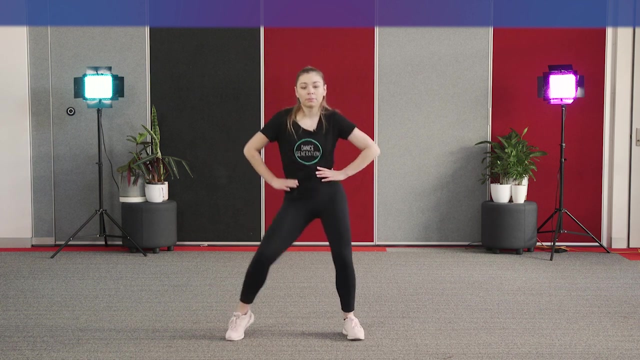 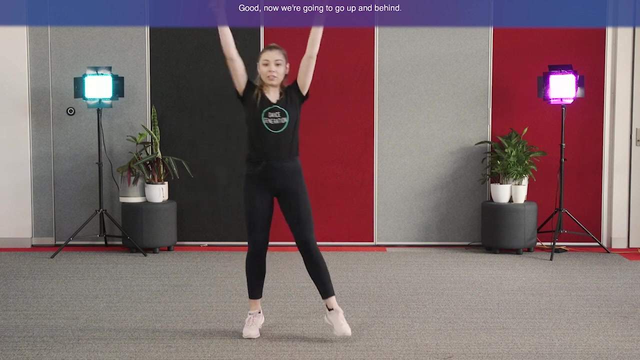 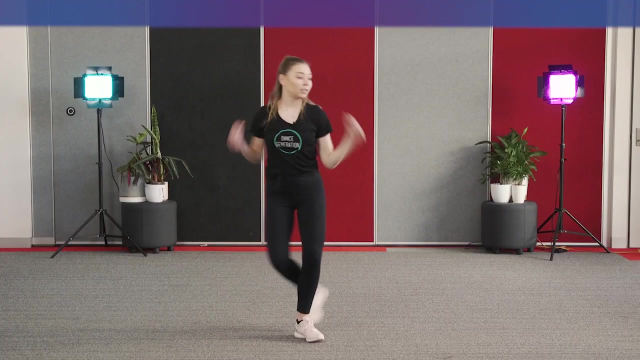 And two, and now one up. good, Good, Now we're going to go up and behind. Look to the side that you're going, And faster. Good, we're going to jump in, cross out, cross fast. 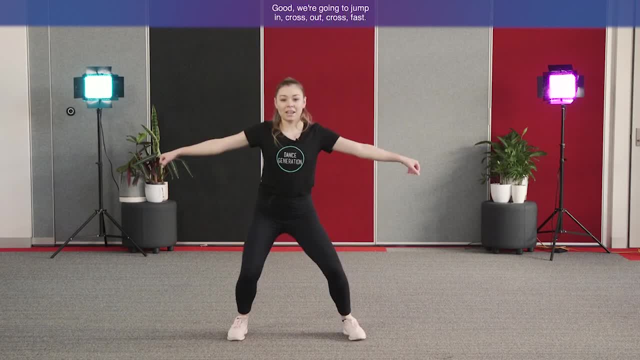 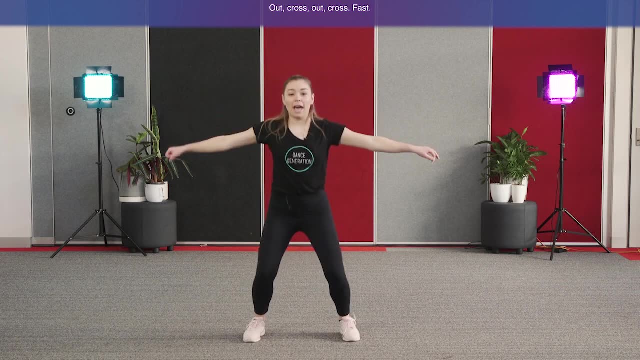 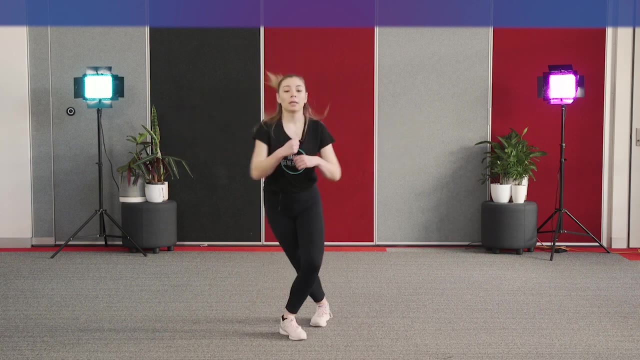 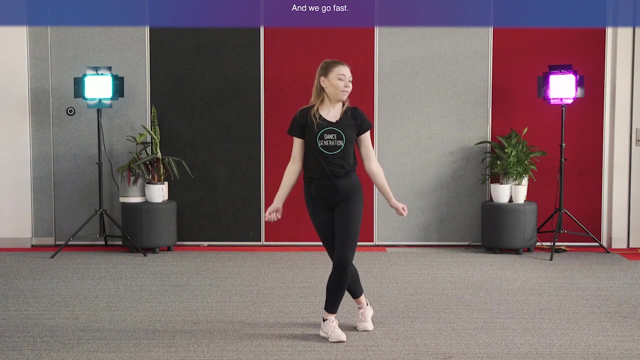 Good, Now we're going to do little circles, Little circles. Good, Now we're going to go up and behind. Look to the side that you're going and faster. Good, Out, cross, Out, cross fast, Up behind, Up behind, And we go fast. 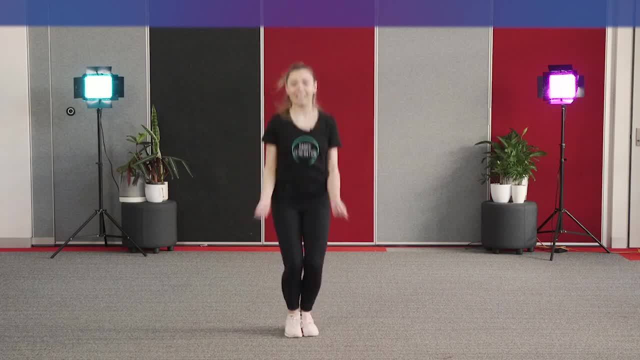 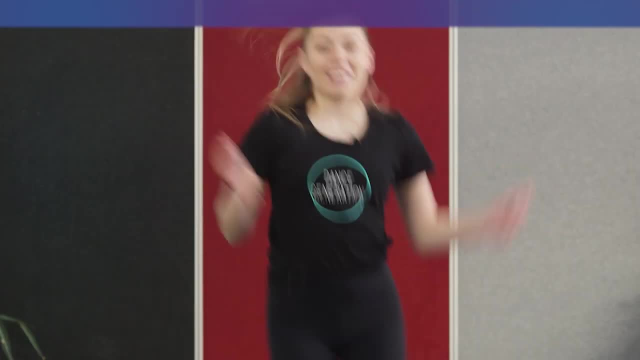 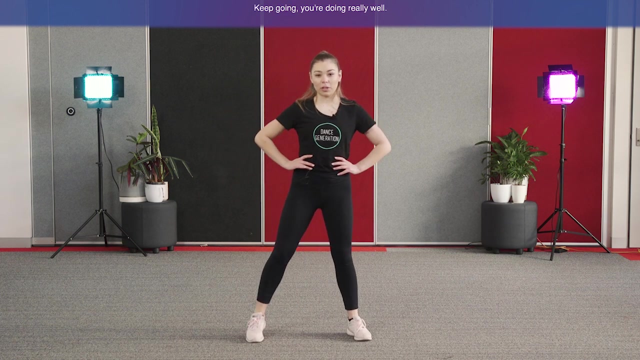 Good, Now we're going to jump like we're skipping rope And side to side. Good work everyone. Keep going. We're doing really well. We're going to do our heads Up, middle and down. Let's go. 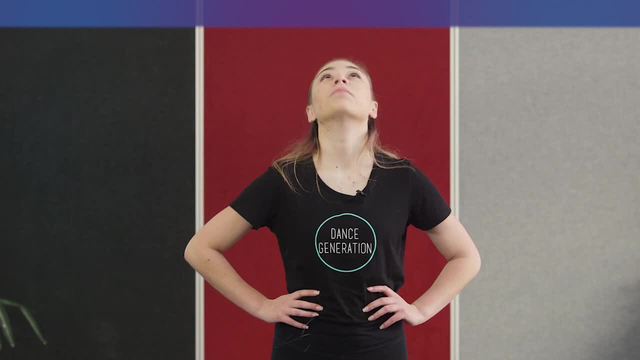 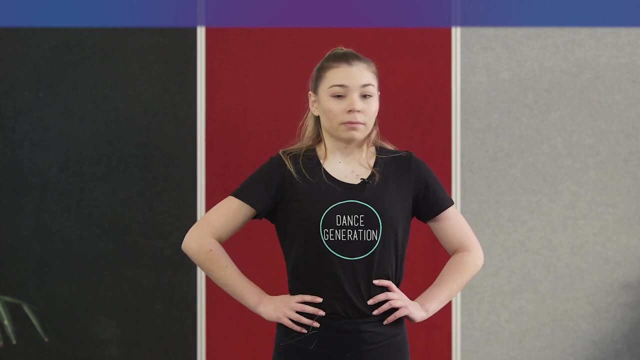 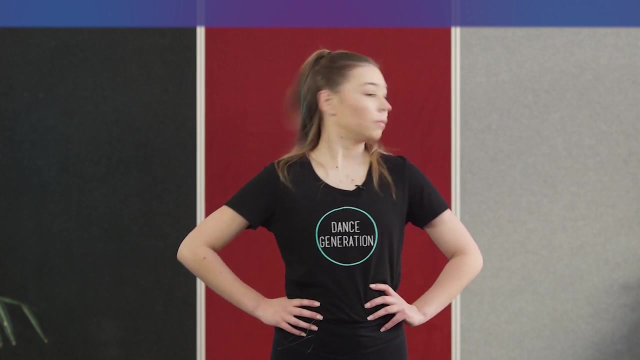 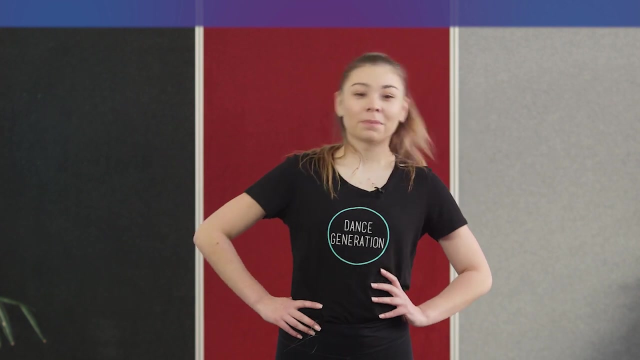 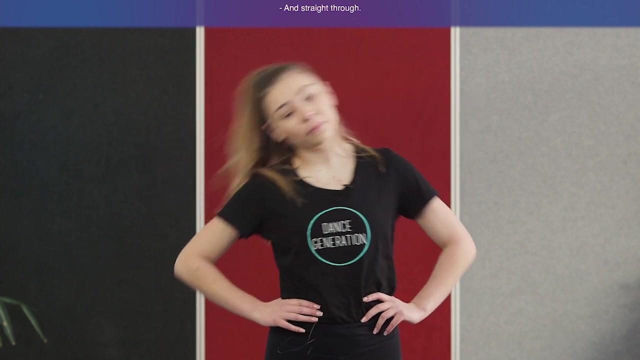 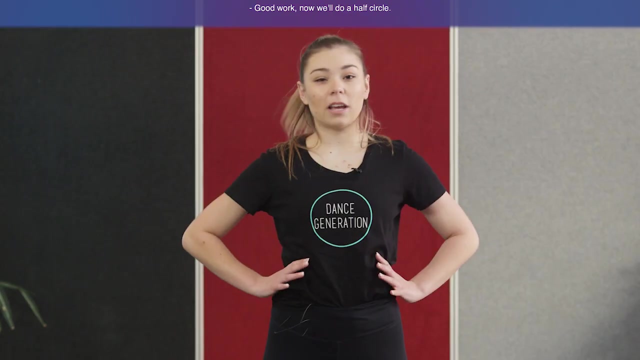 Let's go straight through Good. Now we're going to go side to side, And don't forget about the middle. Straight through Good Now. this time we're going to get that ear to our shoulder And straight through Good work. Now we're going to do a half circle. 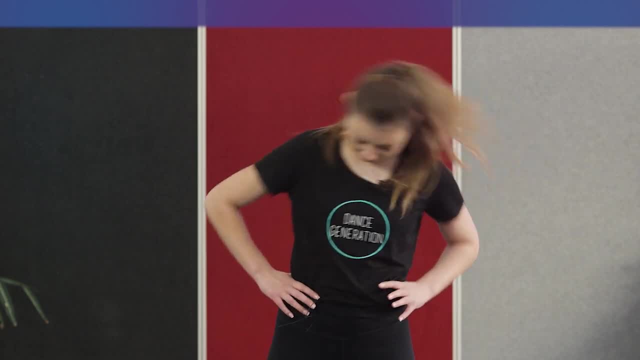 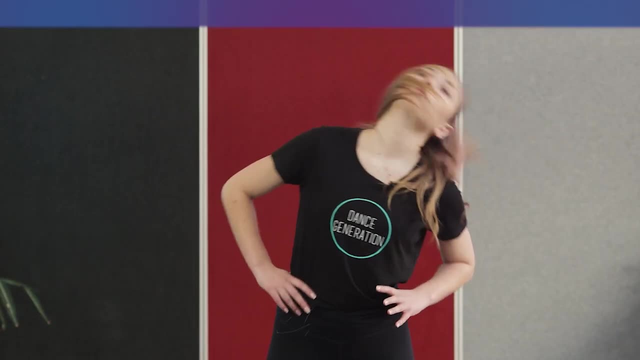 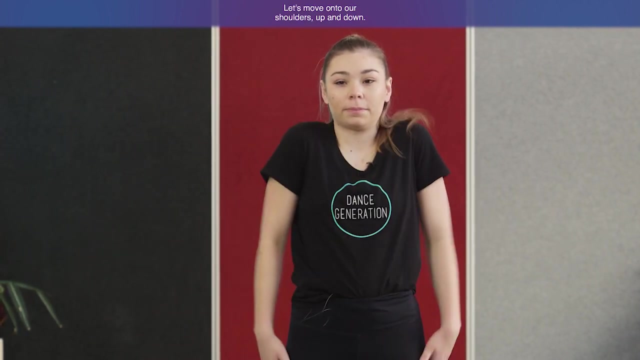 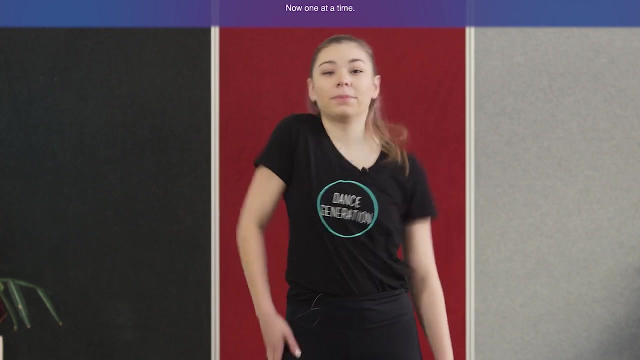 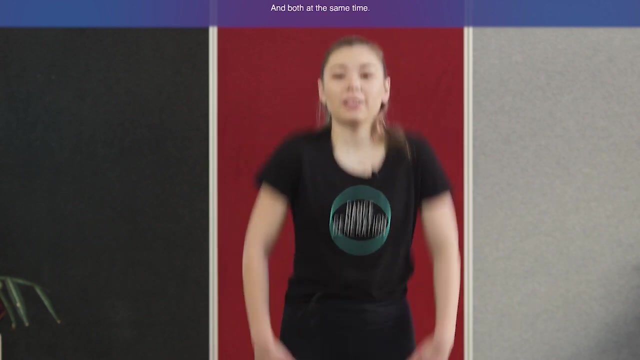 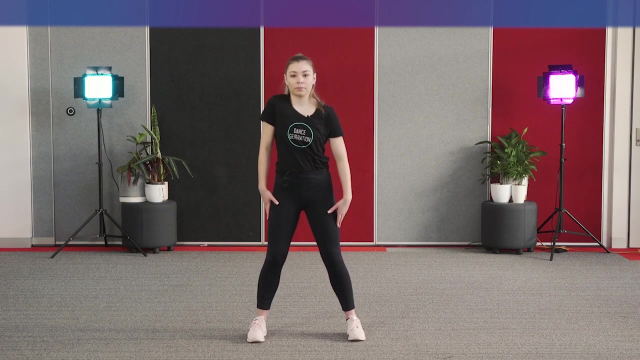 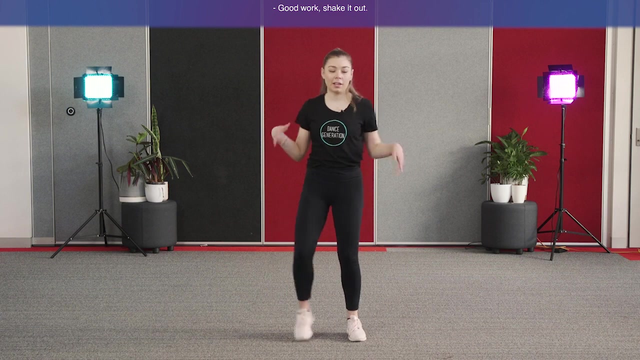 Let's do a full circle Other way, Good. Let's move onto our shoulders Up and down Now, one at a time And by the same time, And one And back And forward, and back, and forward, back forward. Good work. Shake it out, Shake out those legs. Good work. 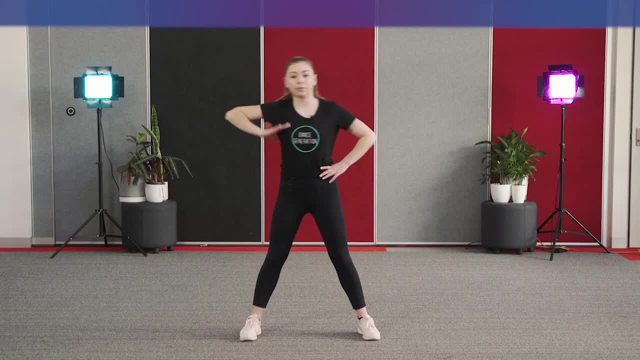 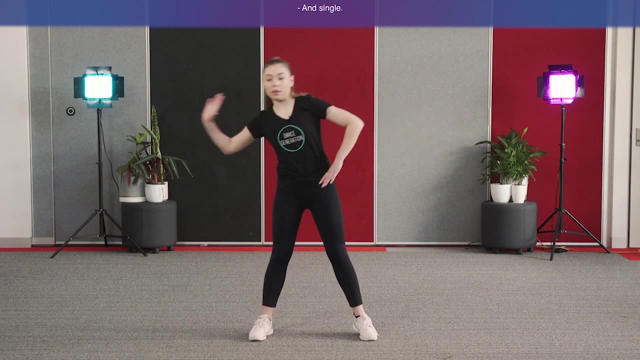 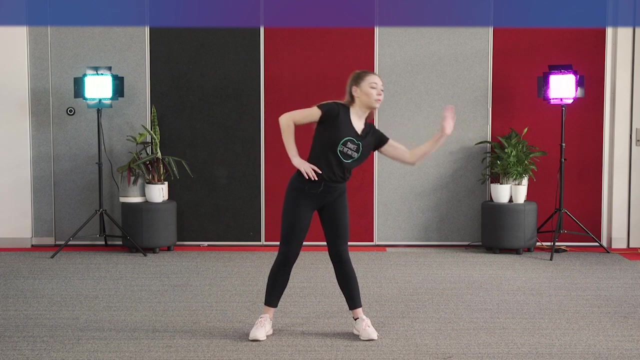 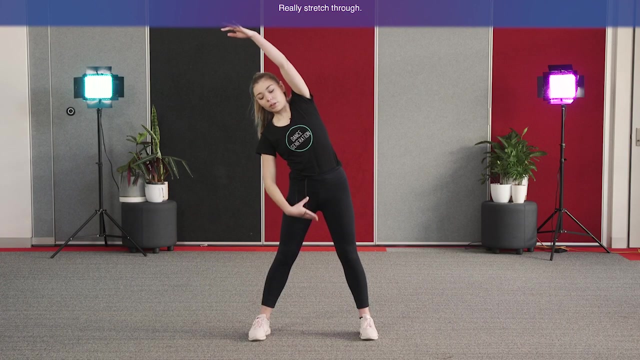 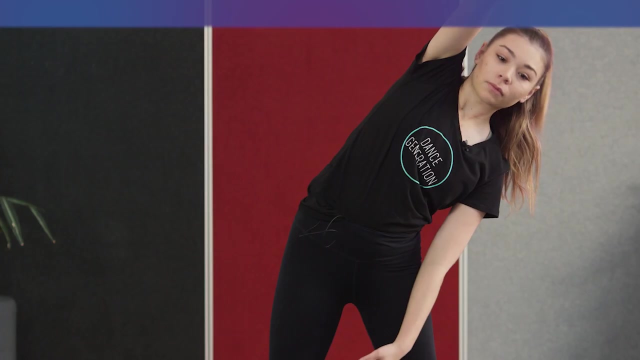 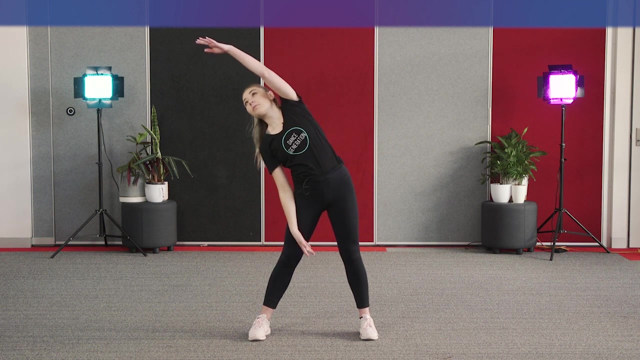 Now we're going to reach side to side. Let's go Push and double and single. Really stretch out those sides and double, Two more doubles. Good Breathe over your head. Really stretch through Other side. Hold it for four now. 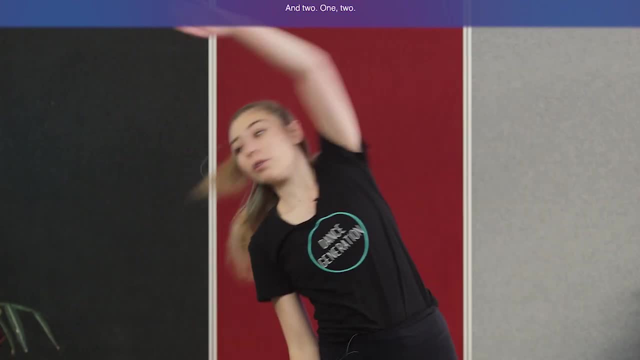 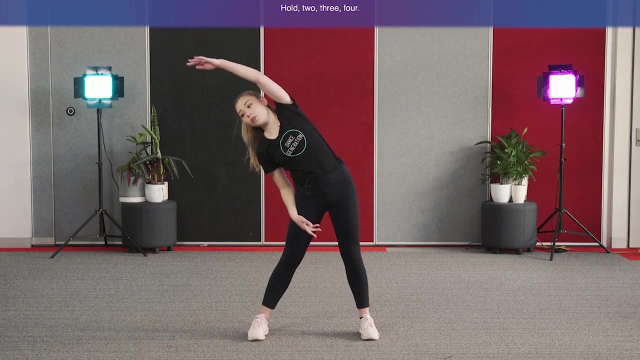 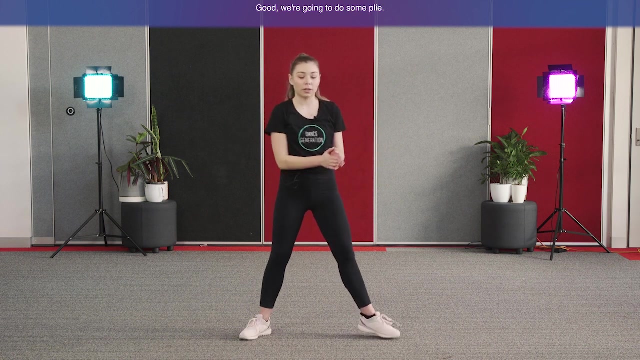 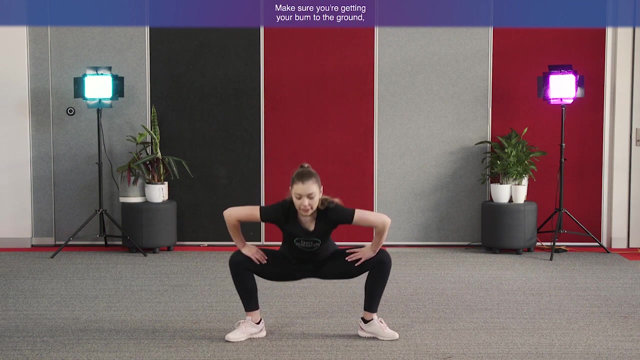 And two, One, two. Hold Two, three, four. Hold One, two, three, four. Good, We're going to do some plie. Good job, Make sure you're getting your bum to the ground, Not keeping it up in the air. 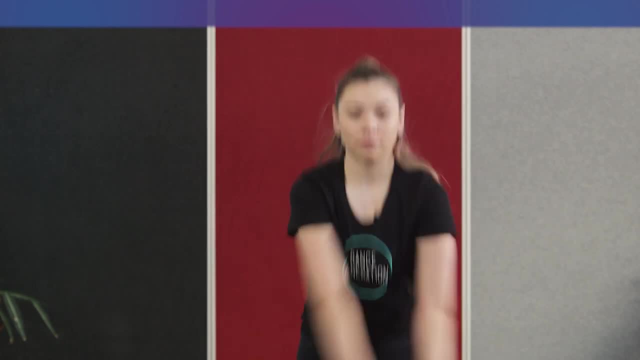 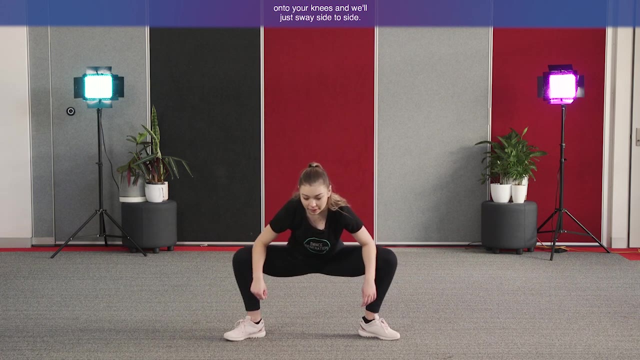 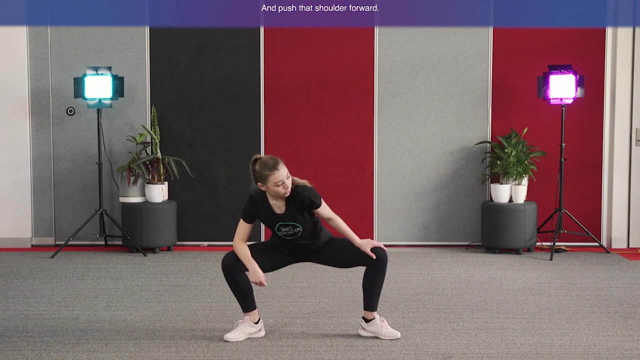 And we're going to hold it down. Rest your elbows onto your knees And we're going to do some plie side to side. Give it a go, even if it's a little bit challenging, And push that shoulder forward. Other side. 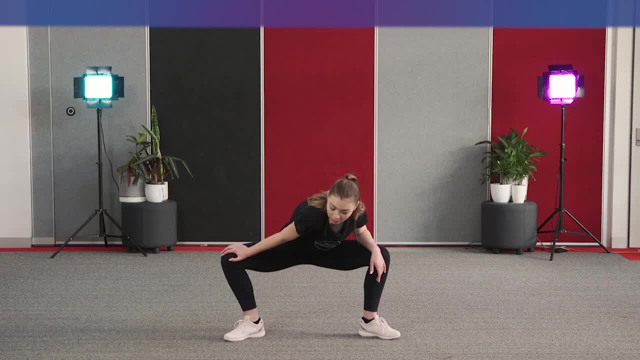 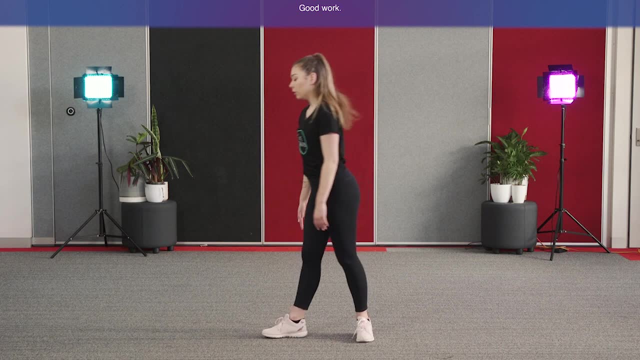 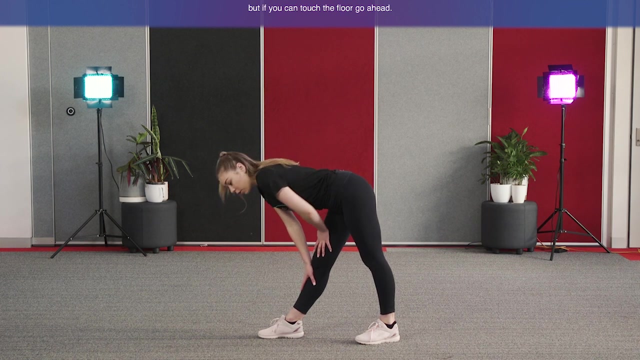 And hold for two, And, And now let's do one more time. Good work, Stretch over to the side. We're going to do our A-frame, So keeping your legs nice and stretched and reaching to your knee. But if you can touch the floor, go ahead. 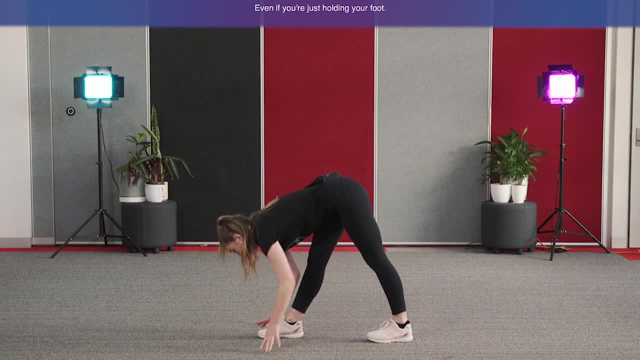 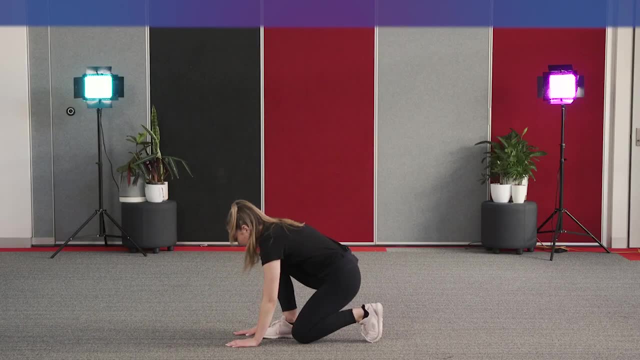 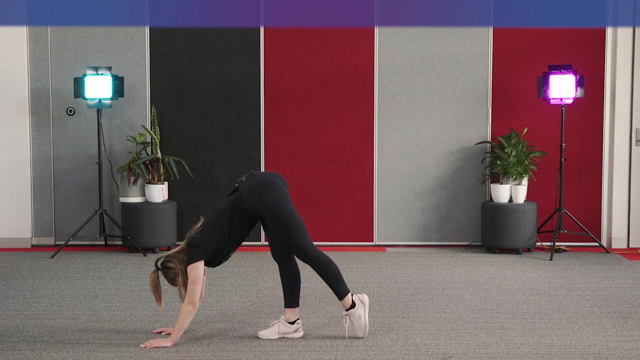 Now we're going to bend and stretch, Even if you're just holding your foot. Good. We're going to get out as far as you can And hold up, And we're going to reach forward And we're going to lunge. 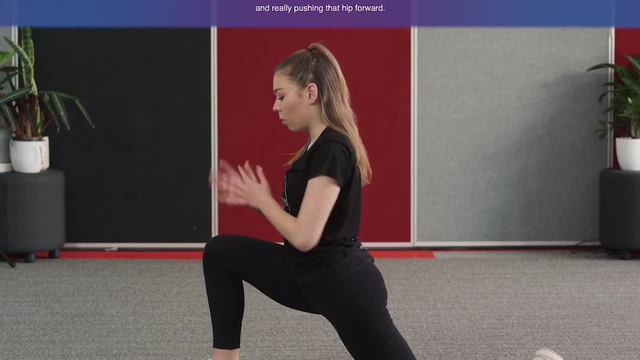 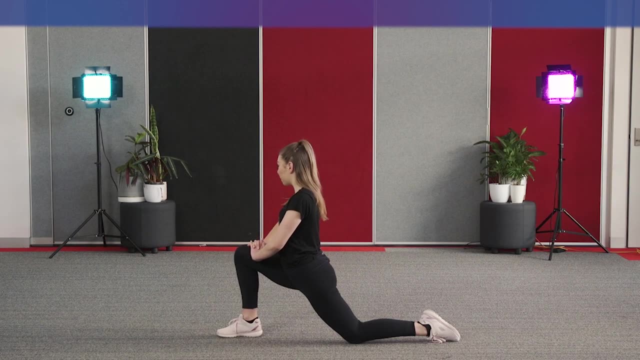 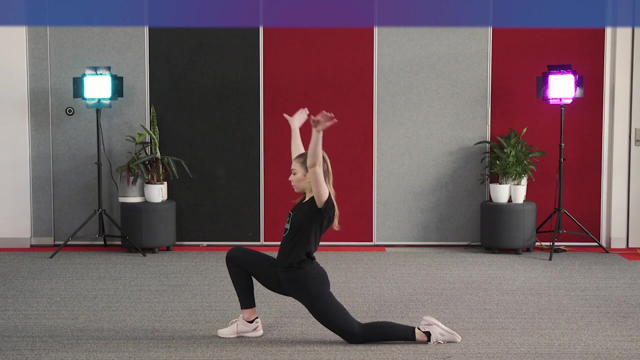 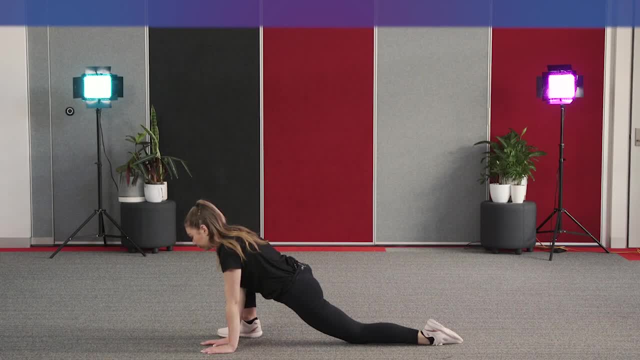 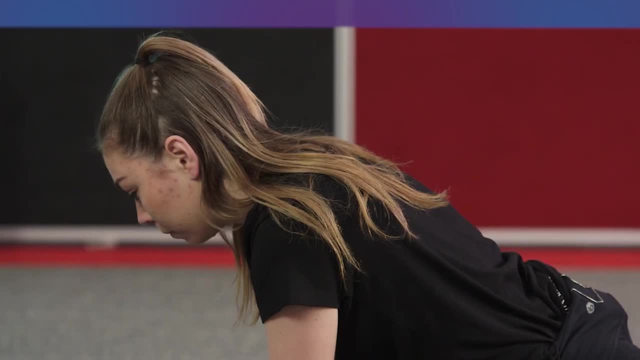 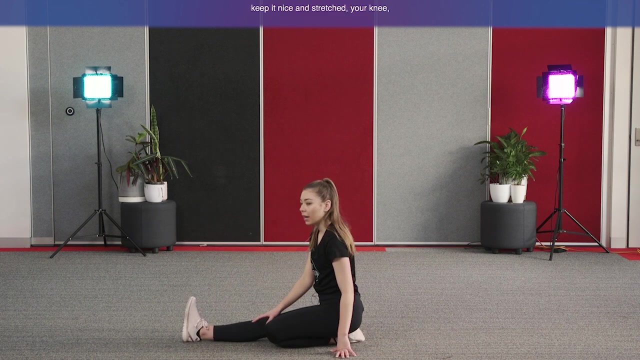 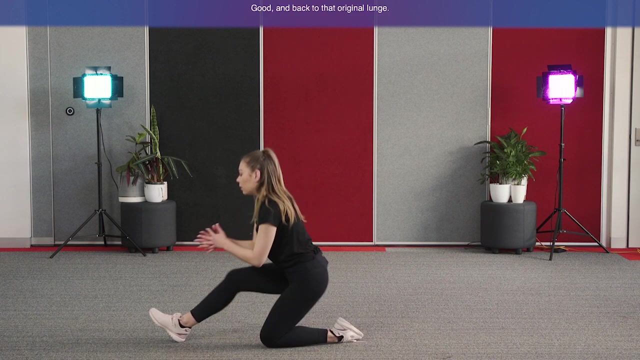 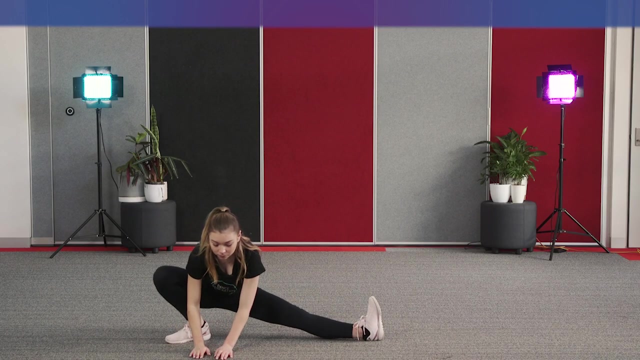 hip pushing forward. You're going to really touch your toes at this stretch. keep it nice and straight your knee and flex that foot up to the roof and try and get that heel off the ground and reaching forward Good, and back to that original lunge and then we'll twist to the front and then to 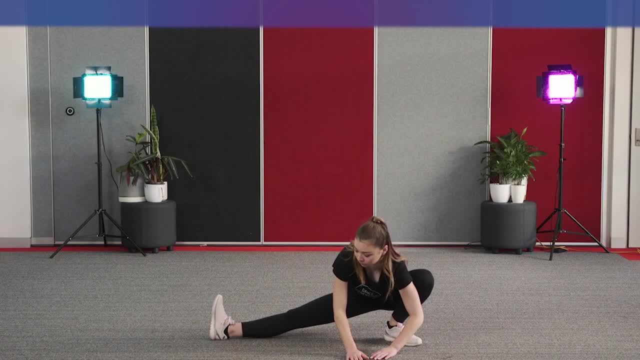 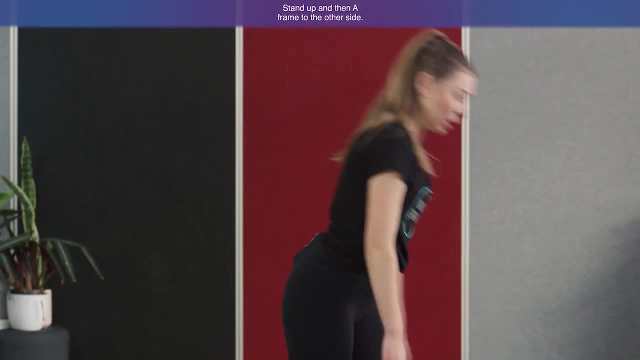 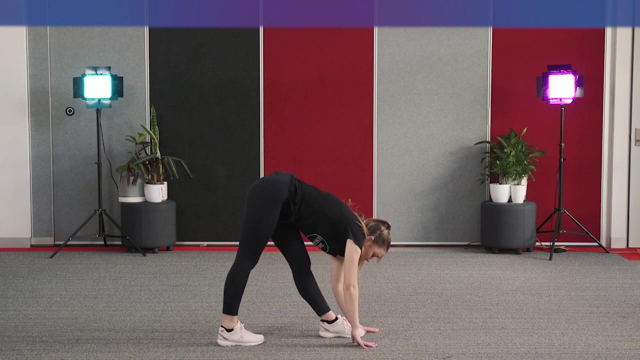 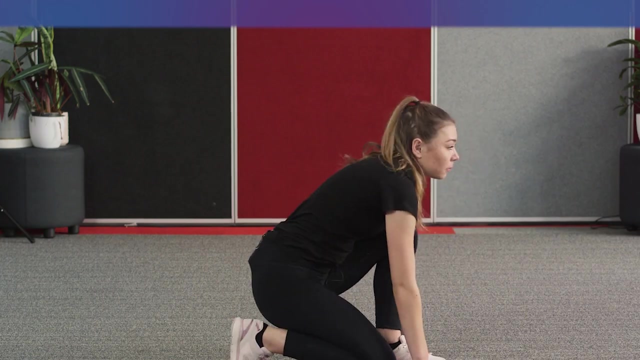 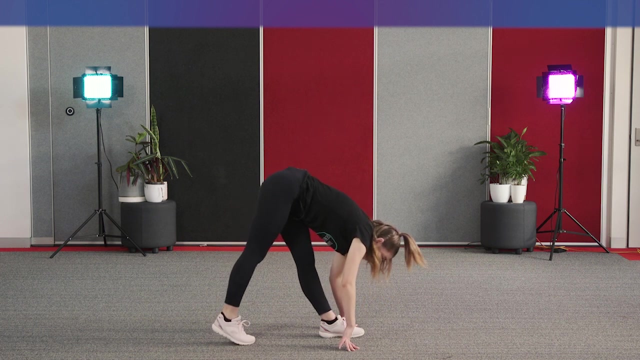 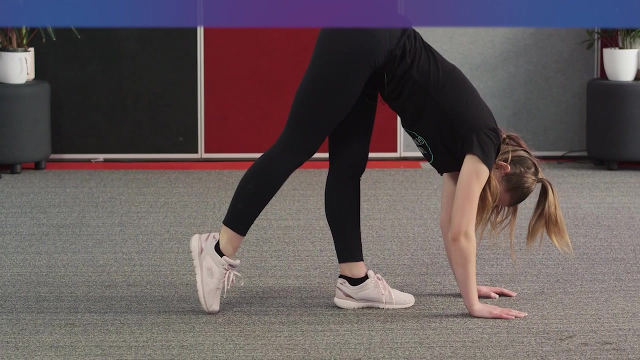 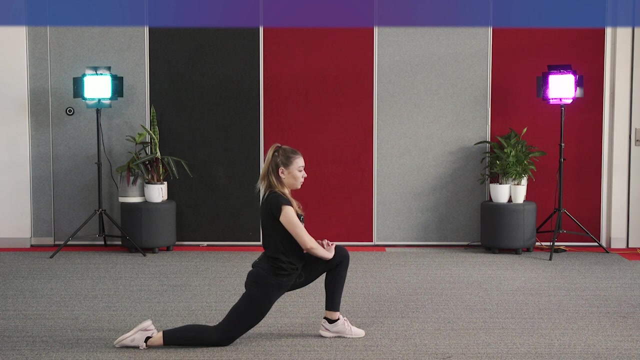 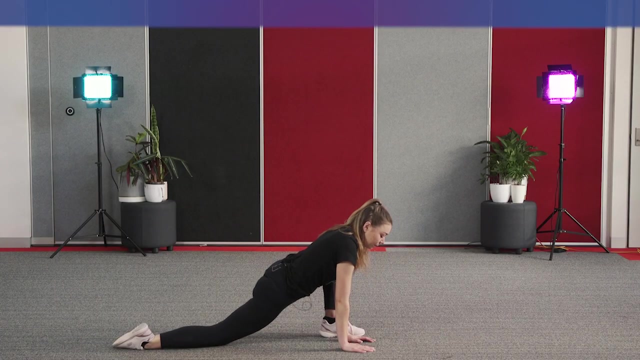 the other side. Good work, Get up, sit up and then A-frame to the other side, Stretching where you're comfortable, And we're going to bend and reach forward and we're landing it forward And we're going to do the lizard stretch. so keep both hands on the floor, keeping those. 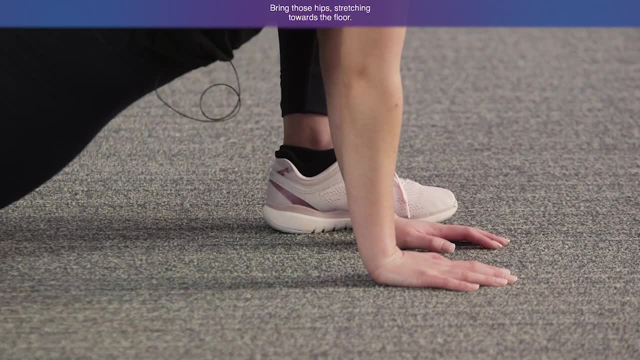 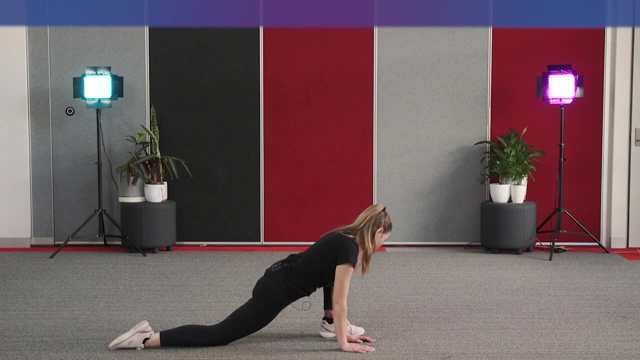 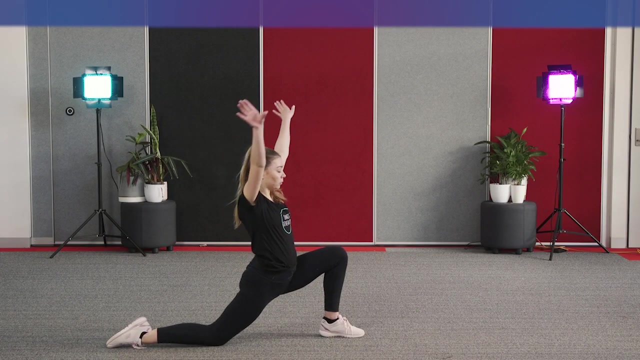 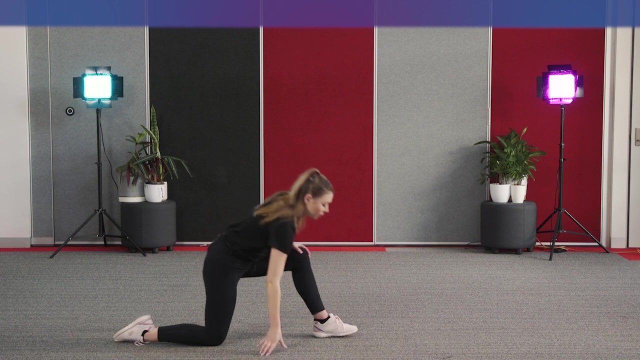 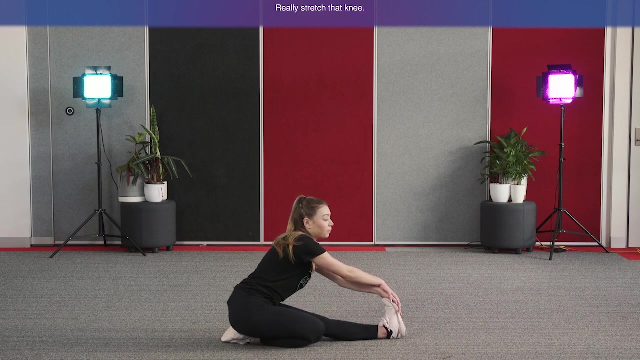 hips stretching towards the floor And back up. Don't forget about your arm stretch. We're going to bring that hip down to the floor, Sit bend, and we're going to swing our arms down. Good, and we're going to go down. 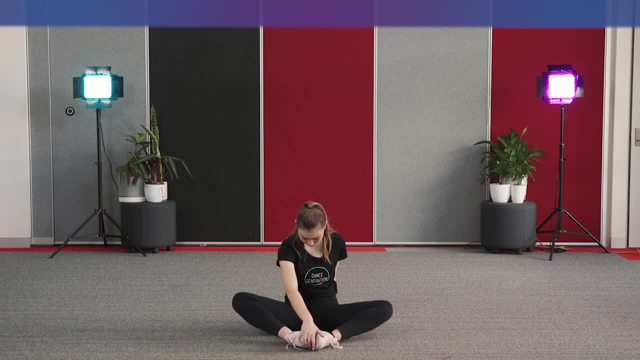 And we're going to start with our legs. so I'm going to start it with the butterfly position And we're going to swing it back and then we're going to do it front. So we're going to sit up, sit down and we're going to lift up our legs. 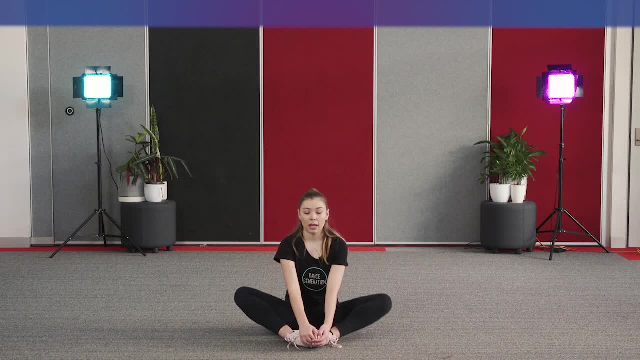 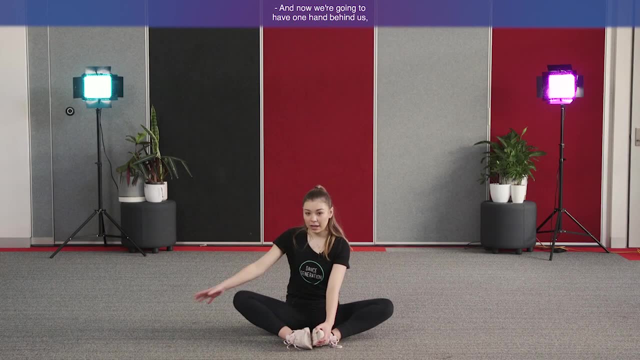 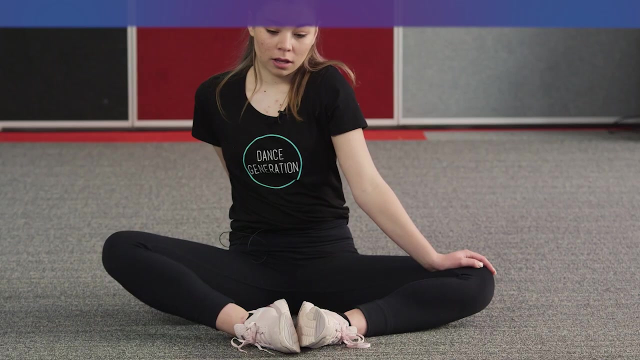 Good, Good, Good, And sitting up nice and tall. And now we're going to have one hand behind us, Keep us sitting up nice and straight, And we push down that knee as far as we can And try the other side. 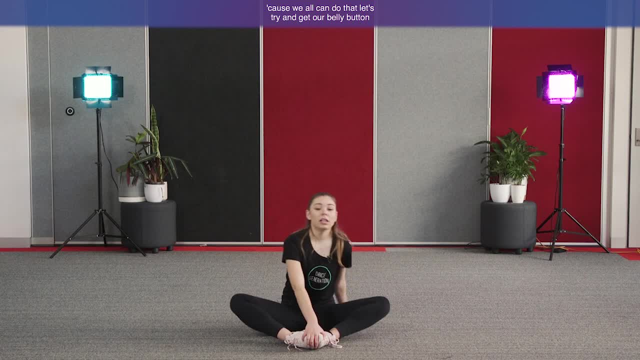 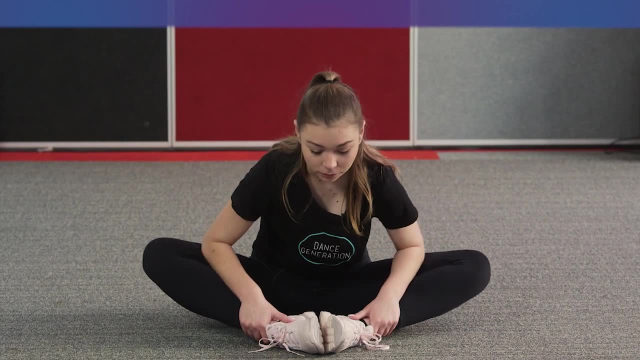 Now, instead of getting your head to your toes- because we all can do that- let's try and get our belly button to our heels. So reach forward and this will give you more of a stretch. And looking straight ahead, in front of you, down the floor. 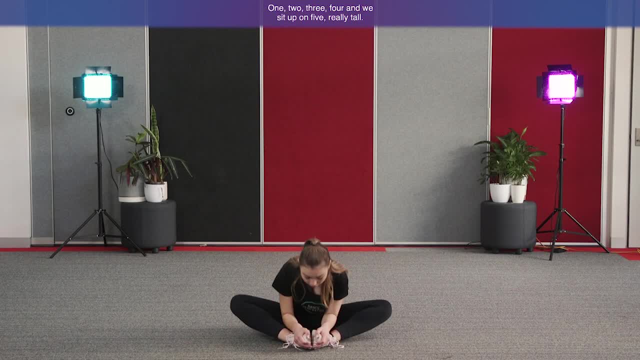 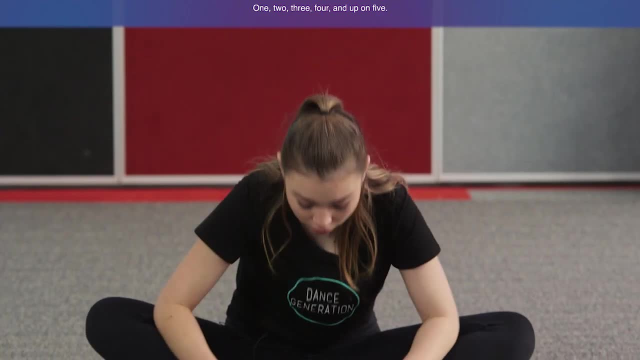 And now we're going to do pulses: One, two, three, four, And we sit up on five, really tall. Let's try it again two more times: One, two, three, four And up on five. Let's try it one more time. 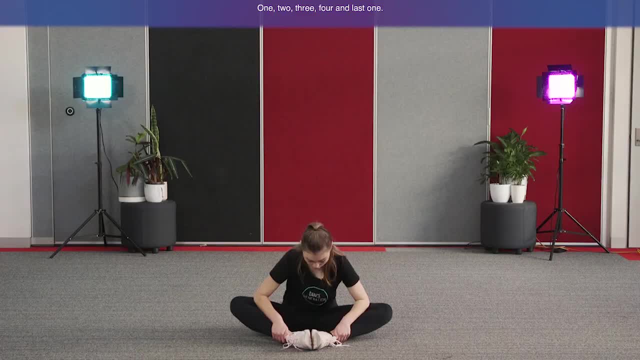 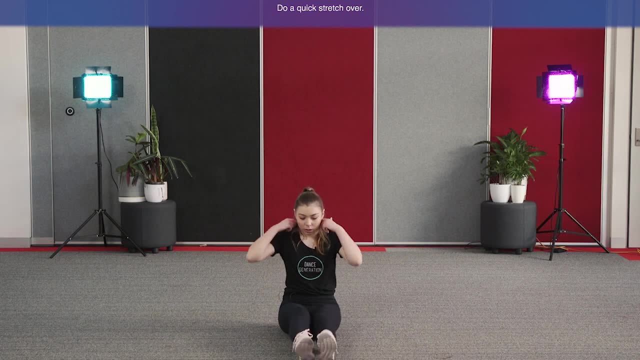 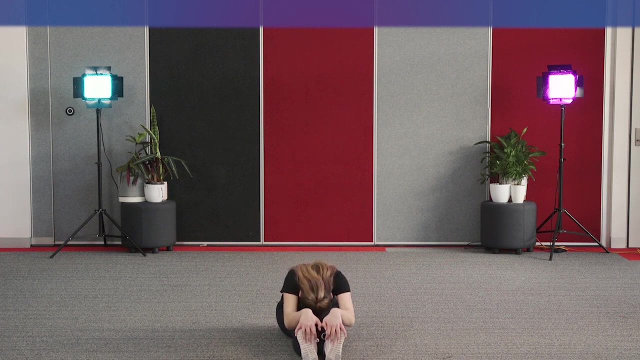 One, two, three, four And last one Good stretch, Shake it out, Shake those legs, Do it quick, Stretch over And keep your head down. Good, Bring that knee in nice and tight And sitting up nice and tall. 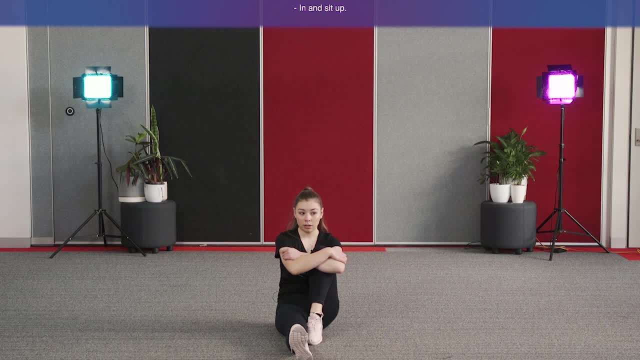 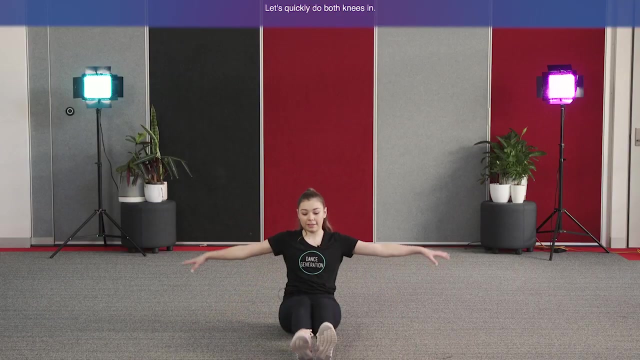 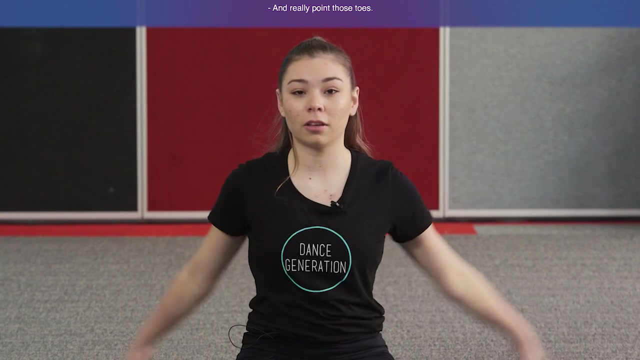 And stretch In And stretch up, Bring it in In, Stretch up Camel. And last one: Good, Let's quickly do both knee dips, Keep it up nice and tall And really point those toes. One more Good work. 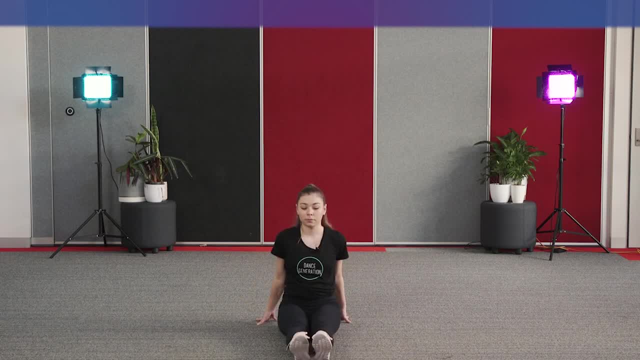 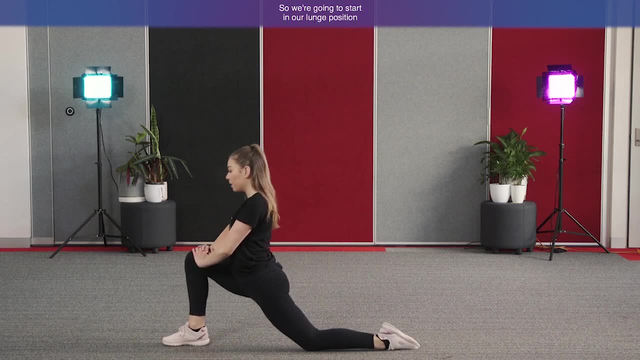 Now, if you can do the splits, give it a go anyway. So we're going to start in our lunge position, like we were before nice, and tall with our backs, Keeping those hips towards the floor. Now, if you're not able to do the splits, give it a go anyway. 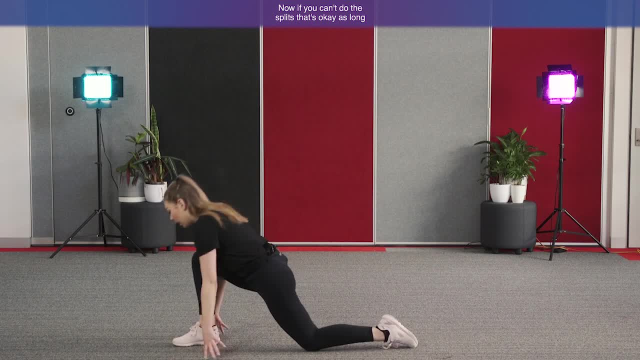 So we're going to start in our lunge position, like we were before Nice, and tall with our backs, Keeping those hips towards the floor. Now, if you can't do the splits, that's okay, as long as you have stretched legs like that. 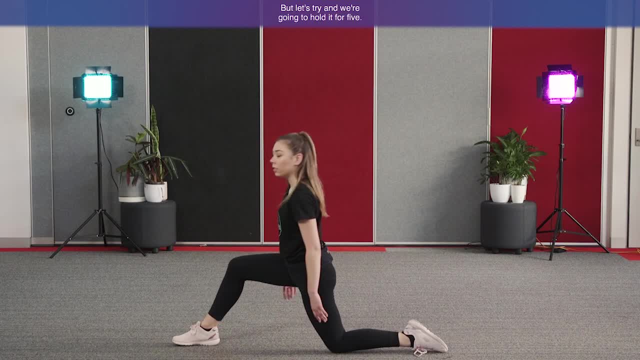 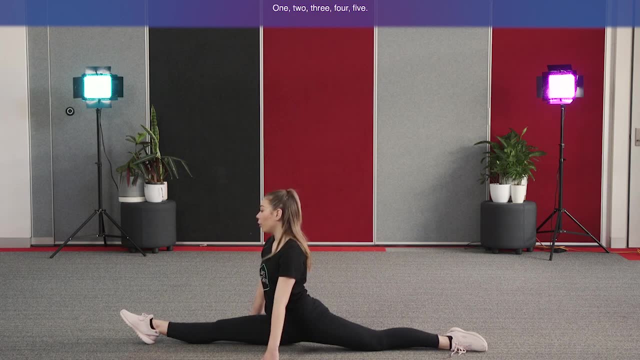 As long as our knees are nice and straight, that's all that matters. But let's try, and we're going to hold it for five Camp. Let's go Stand up nice and tall. One, two, three, four, five. 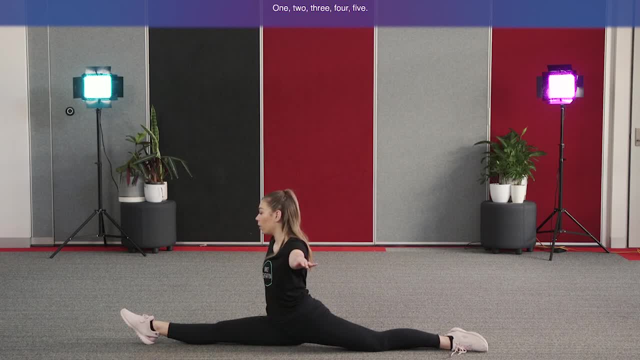 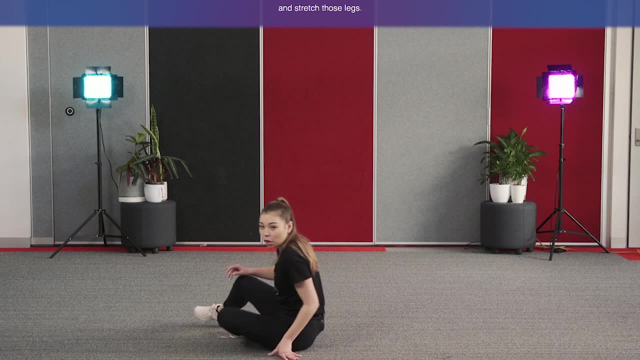 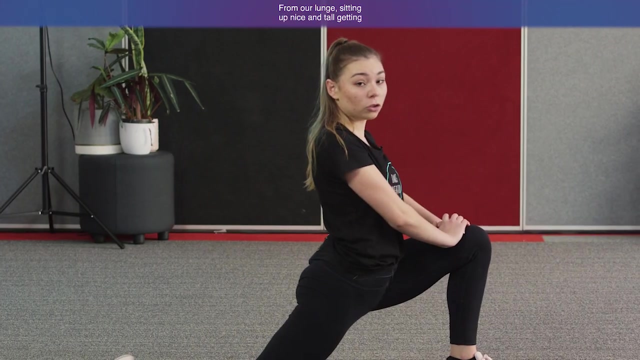 And if you can hold without your hands one, two, three, four, five, Good work. Bring that leg around and stretch those legs. Let's do our left leg from our lunge. Stand up nice and tall, keeping those hips towards the floor. 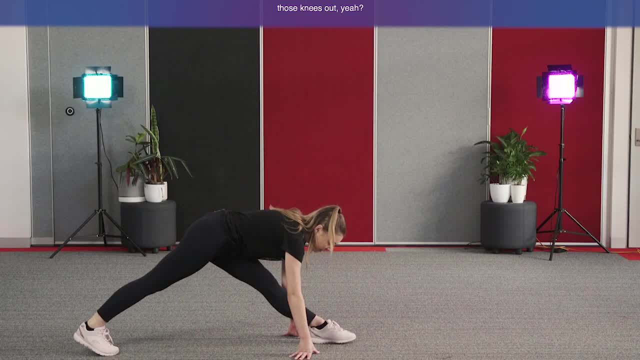 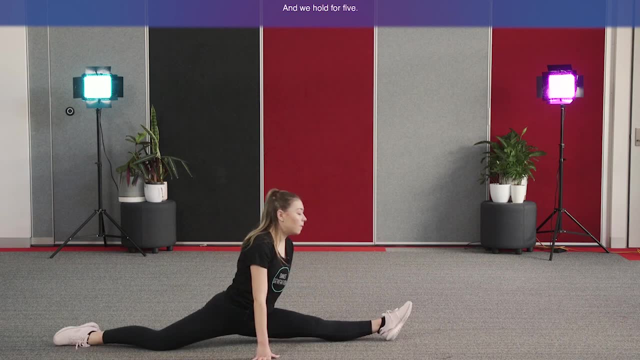 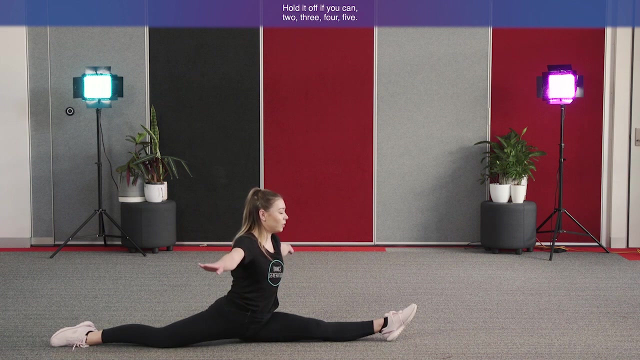 Again, if you can't do the splits, just really stretch those knees out. yeah, from that position, And we hold for five: One, two, three, four, five. Hold it off, if you can. Two, Three, Four. 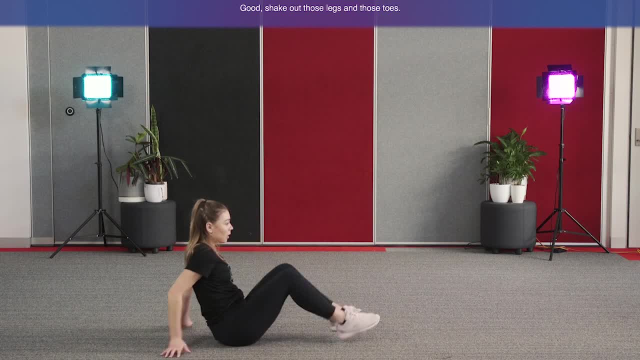 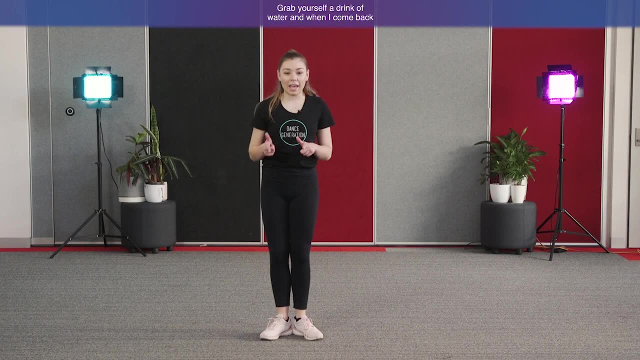 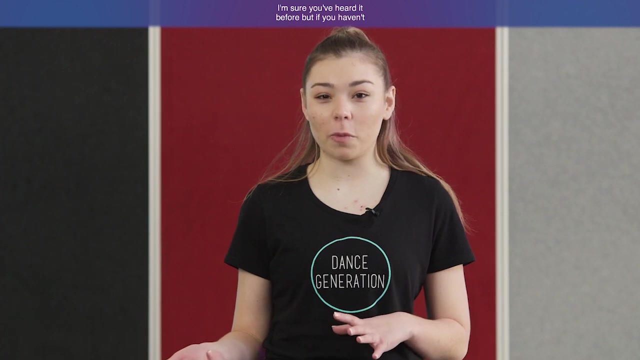 Five And bring it around. Good, Shake out those legs and those toes, Grab yourself a drink of water and when I come back we will start our dance. So today we're going to be doing the song Break Free. I'm sure you've heard it before, but if you haven't, then it's a really fun song. 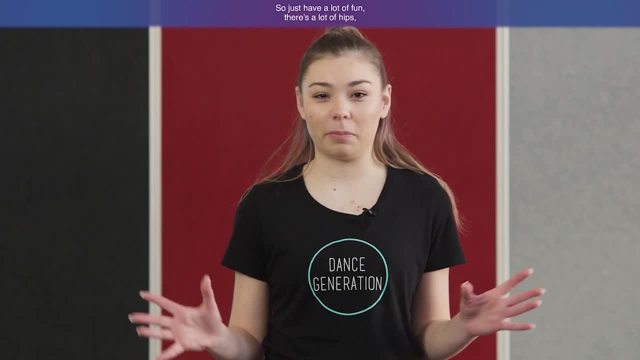 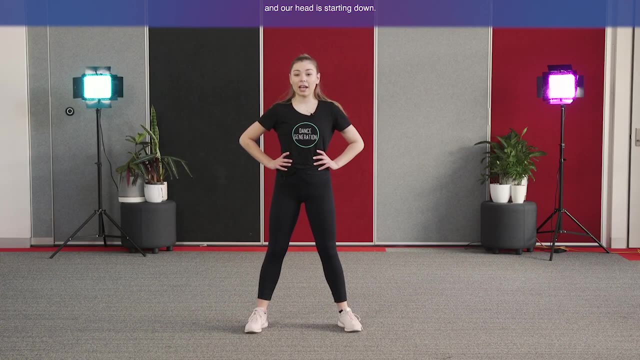 Lots of energy, So just have a lot of fun. There's a lot of hips, You know. have a good time, Don't stress about it too much. Okay, so we start with our feet apart and our head is starting down. 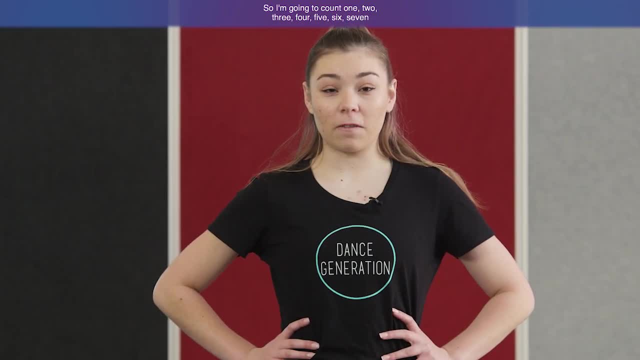 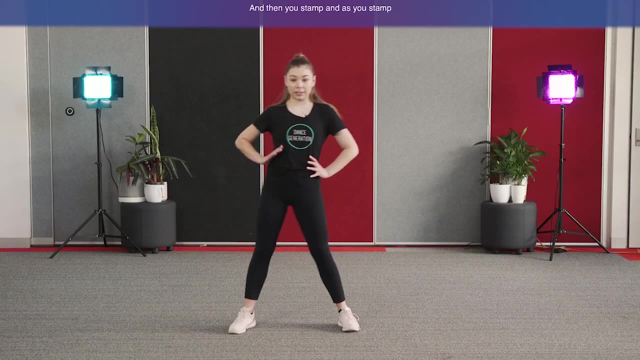 So I'm going to count one, two, three, four, five, six, seven. On eight your head comes up, yeah, And then you stamp, and as you stamp, your hips going to the side that you're stamping. 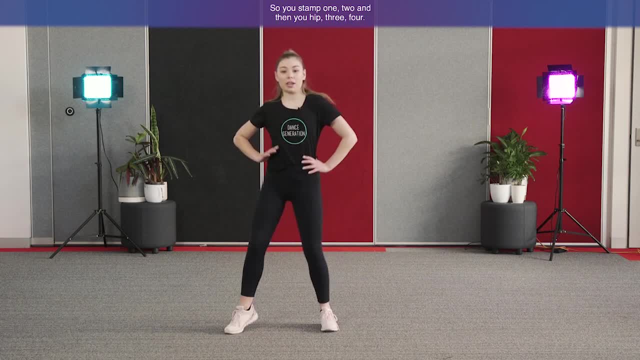 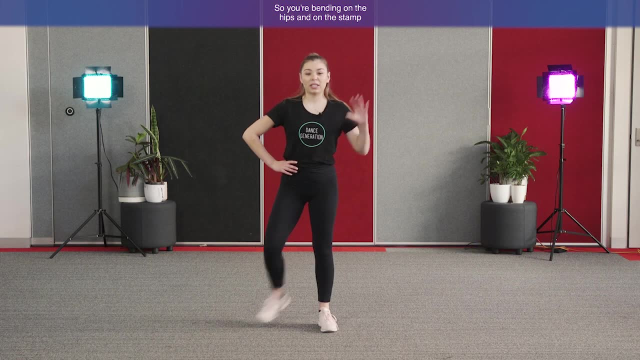 So you stamp one, two, and then you hit three, four, Stamp five, six, seven, eight. So you're bending on the hips and on the stamps. it's really tall. Yes, Let's try that again. So head down. 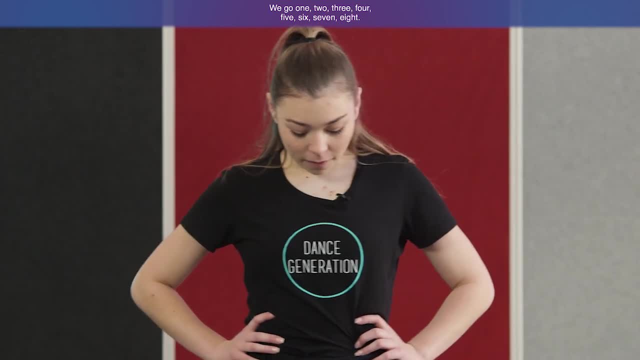 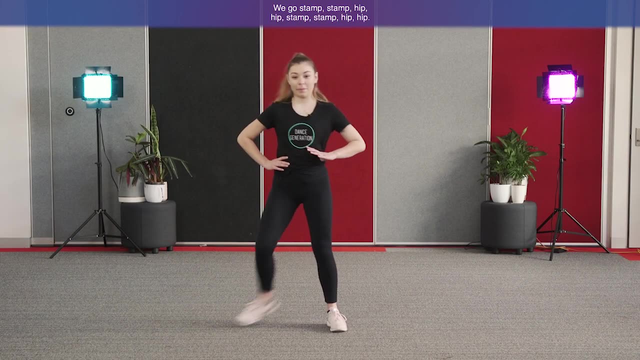 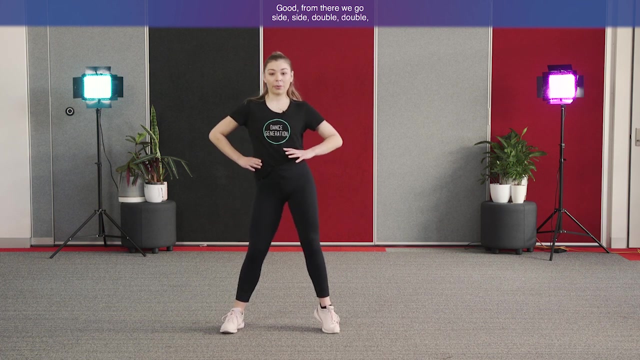 We go one, two, three, four, five, six, seven, eight. We go stamp stamp hip hip, stamp stamp hip hip Good. From there we go side side double double, side side double double. 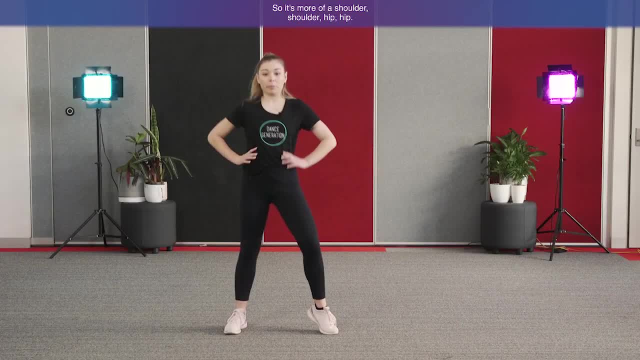 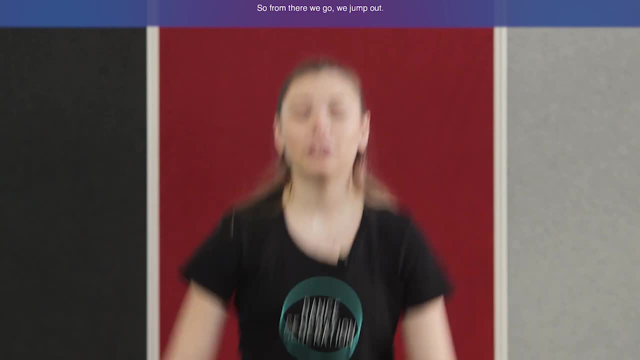 So it's more of a shoulder, Shoulder, hip, hip, shoulder, shoulder, hip, hip. Yes, So from there we go, We jump out. As we jump out, our hands come just to our ribs, So you should be able to feel those ribs in there. 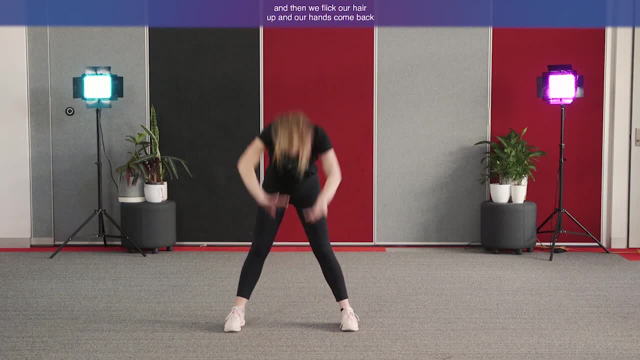 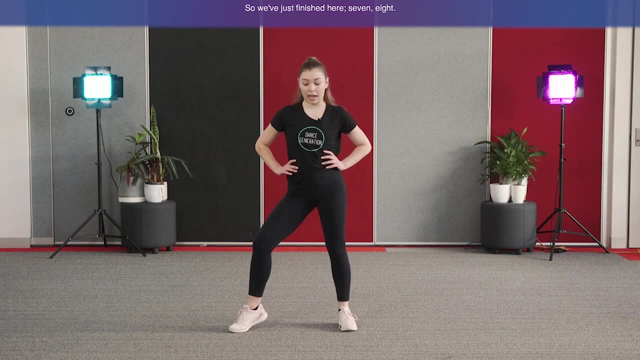 So grab those ribs and then we touch the floor and then we flick our hair up and our hands come back to our hips. Yes, So we've just finished here. Seven, eight, We jump up ribs down flick. 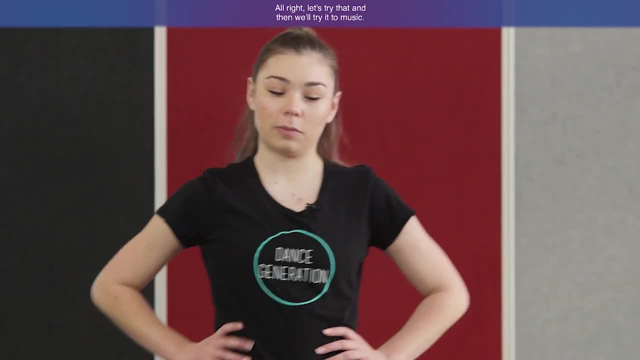 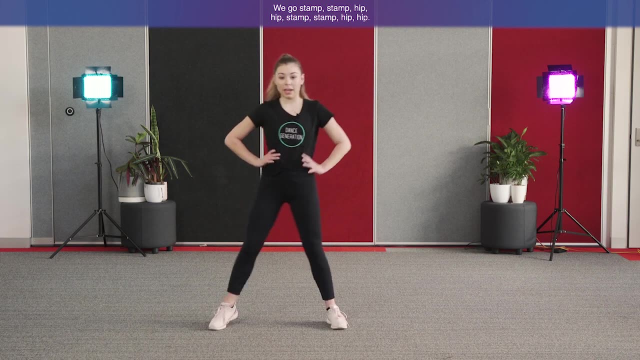 Yeah, All right, Let's try that, and then we'll try it to music. So we go one, two, three, four, five, six, seven, eight. We go: stamp, stamp, hip, hip, stamp, stamp, hip hip. 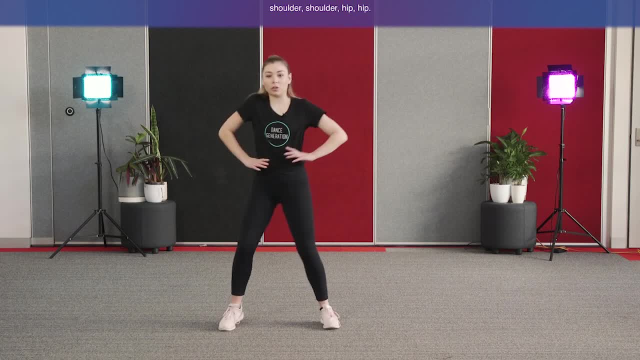 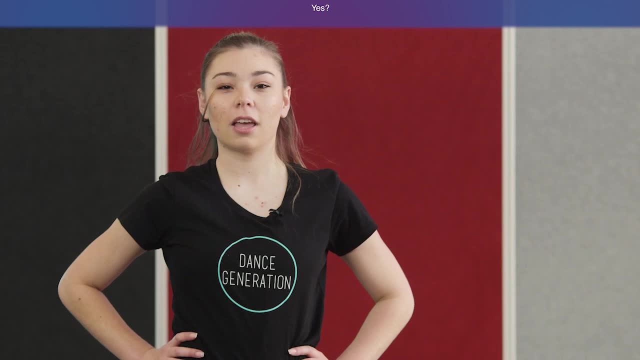 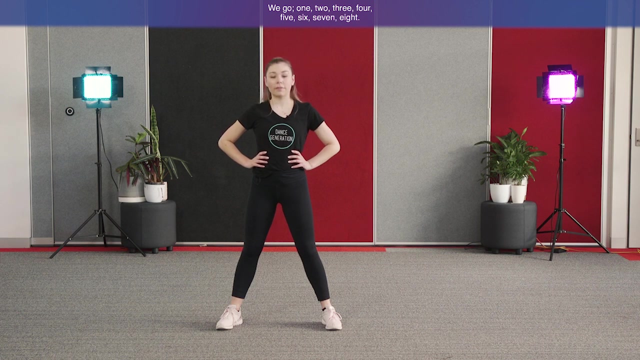 We go: shoulder, shoulder, hip, hip, shoulder, shoulder, hip, hip. We go ribs Jump out Down hips. Yes, One more time, and then we'll try it to music. We go One, two, three, four, five, six, seven, eight. 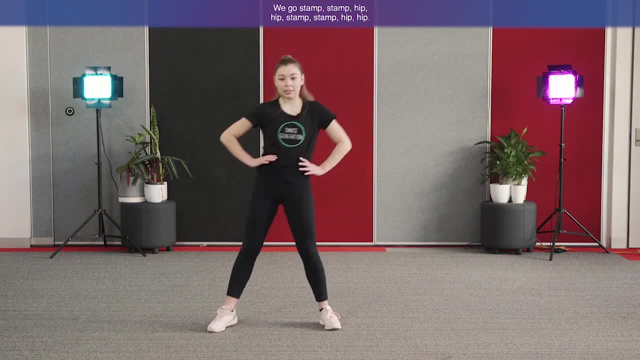 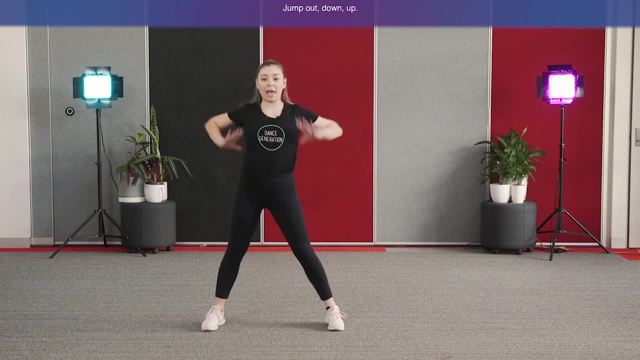 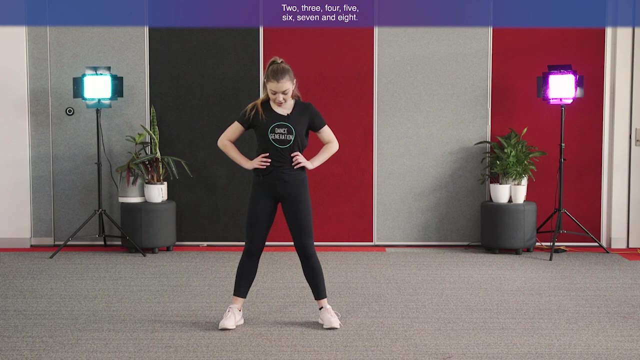 We go: stamp stamp hip hip. stamp stamp hip hip, Shoulder, shoulder, hip hip, shoulder, shoulder, hip, hip. Jump out Down up. Okay, Let's try it to music: Two, three, four, five, six, seven, eight. 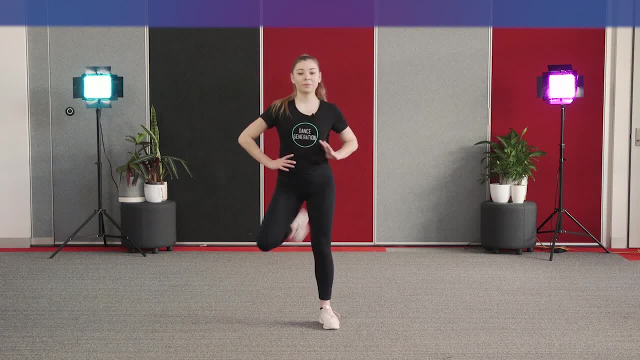 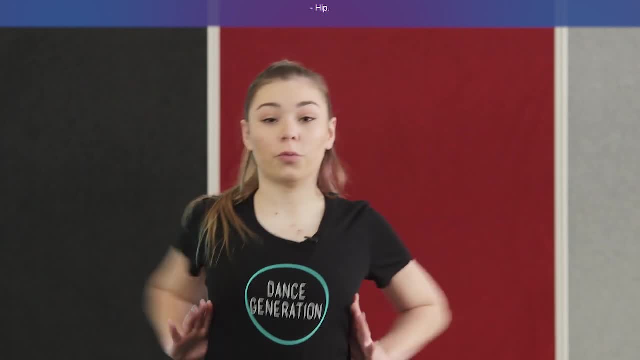 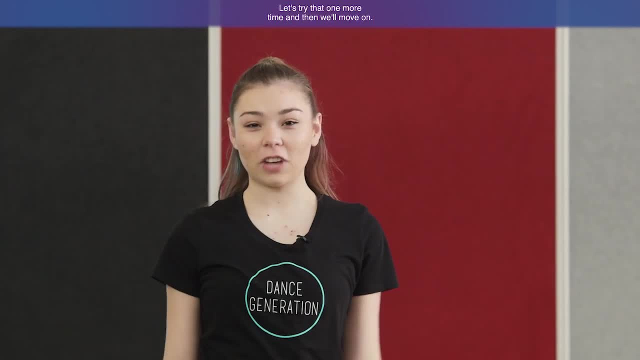 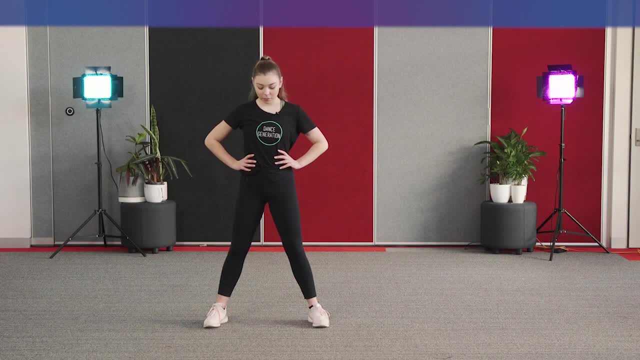 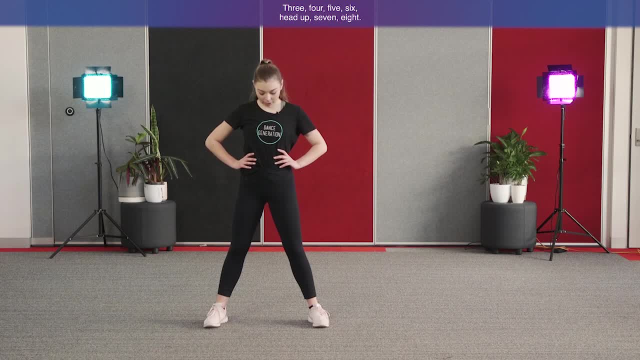 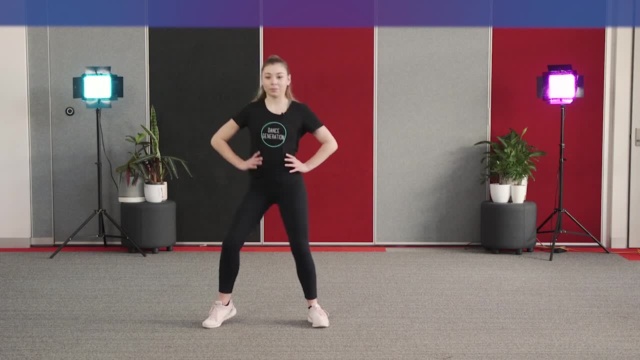 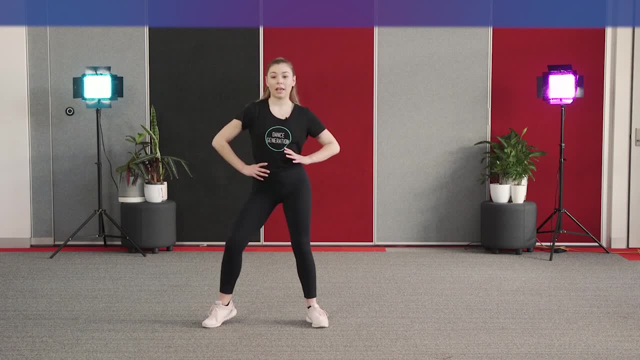 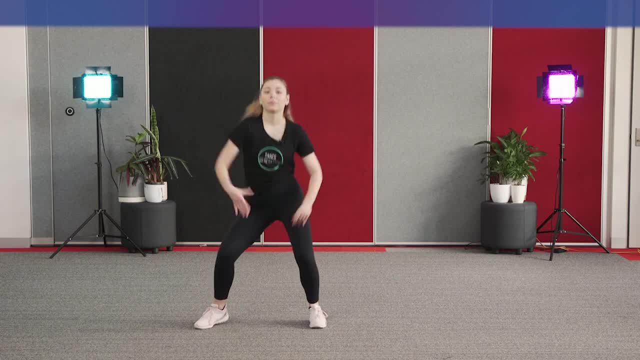 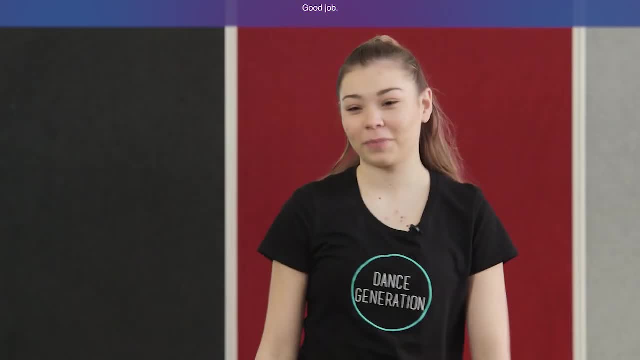 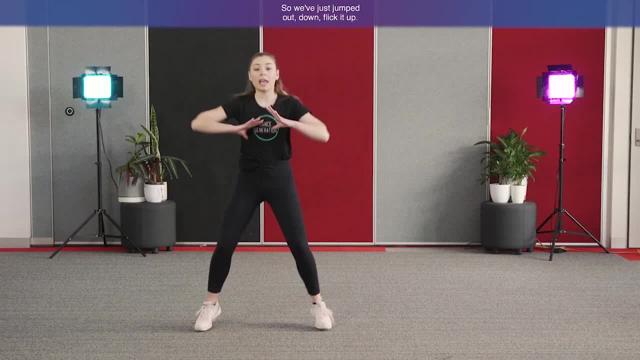 One, two, three, four, five, six, seven, eight. One, two, three, four, five, six, seven, eight. Now we're gonna jump onto our next steps. So we've just jumped out down, flick it up. 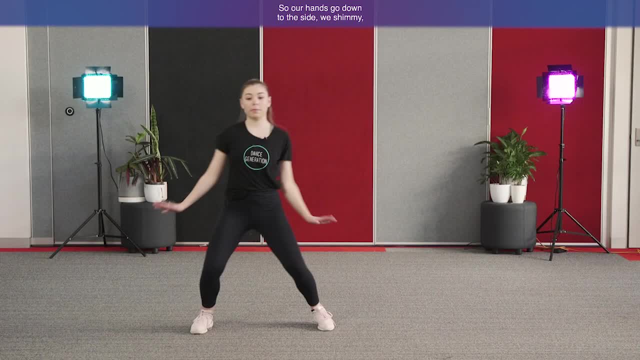 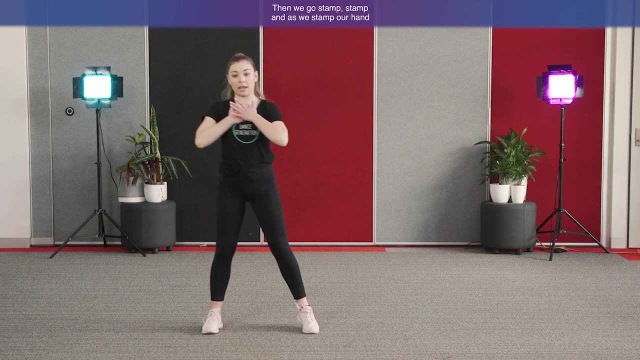 From here we do our shimmy, So our hands go to down to the side. We shimmy, we point our foot, We shimmy, we point our other foot. Then we go, step, step, And as we step, a hand comes over our chest. 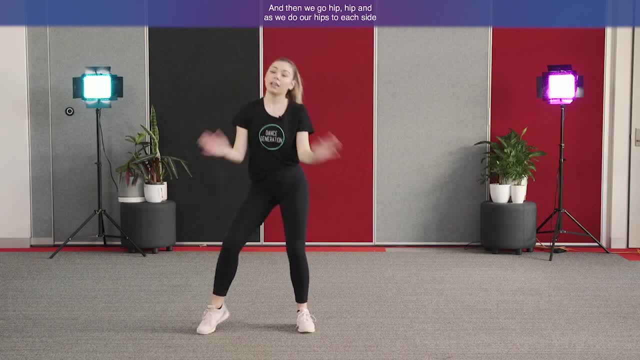 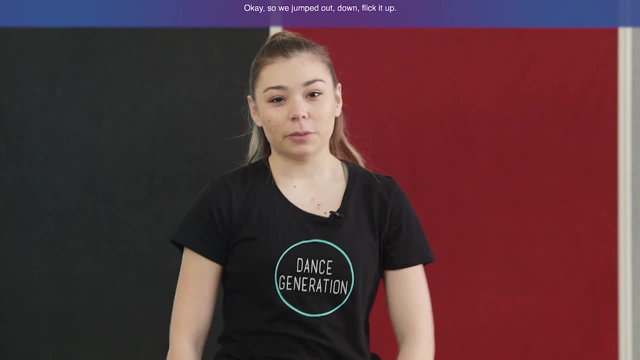 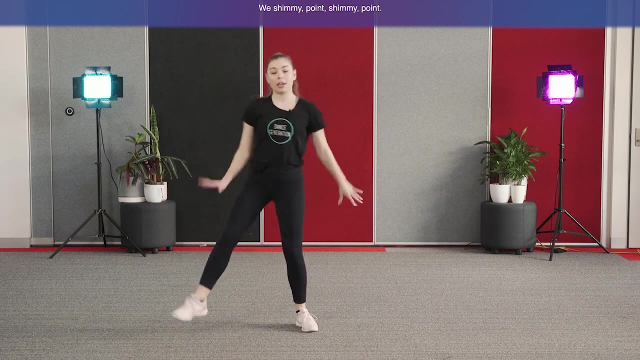 Yes, And then we go hip, hip And as we do our hips to each side, our head goes to the same side that we're jumping. Cool, doing our hips, Okay, so we jumped out down, flick it up. We shimmy point, shimmy point. 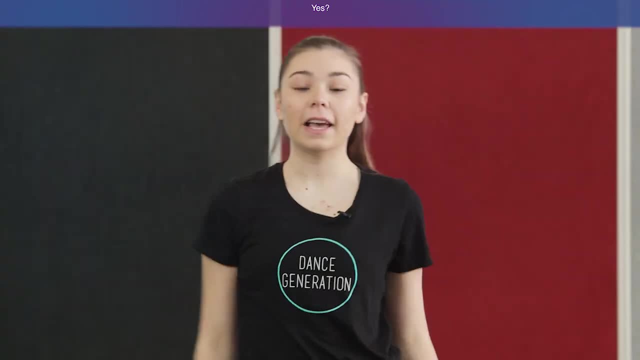 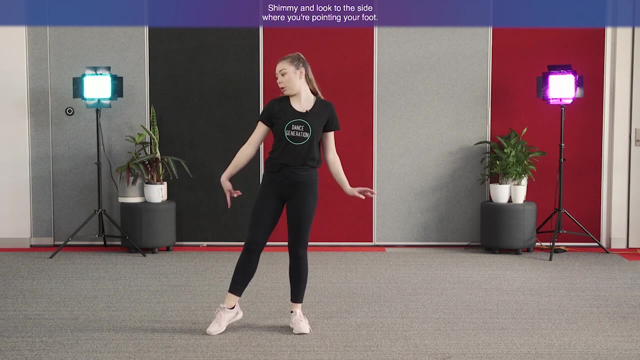 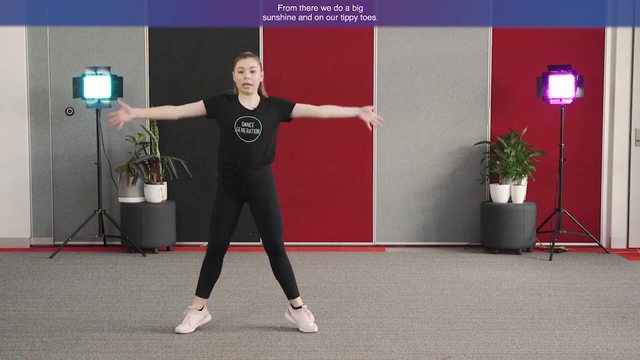 heart, heart, head, head, Yes. and as we shimmy, we point that toe and we look to the side, shimmy, and look to the side where you're pointing your foot- Step, step, hip, hip. From there we do a big sunshine and on our tippy toes, Yes. so we're in second position. 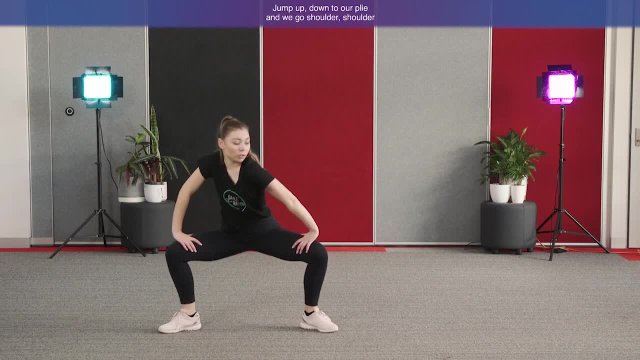 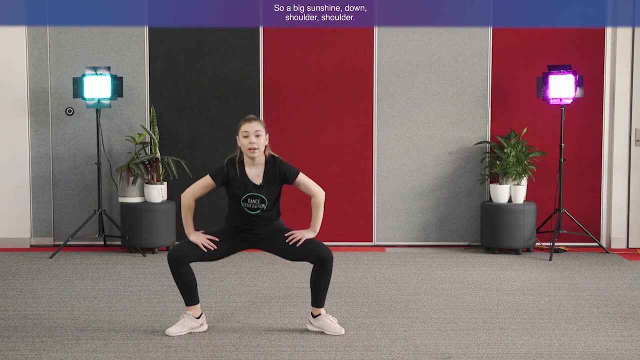 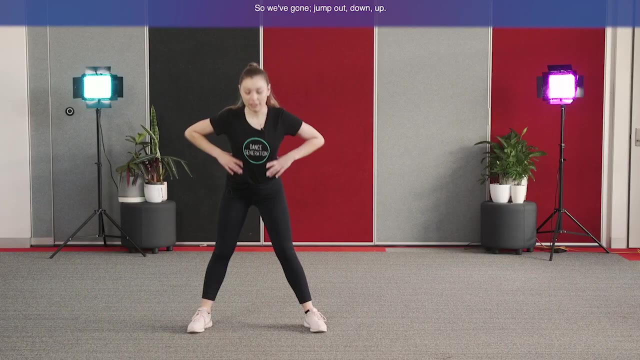 Jump up down to our plie and we go shoulder shoulder and we look over our shoulder as we do it. So big sunshine down, shoulder shoulder. Good, Let's try that all together. So we've gone: jump out down up, We go shimmy. 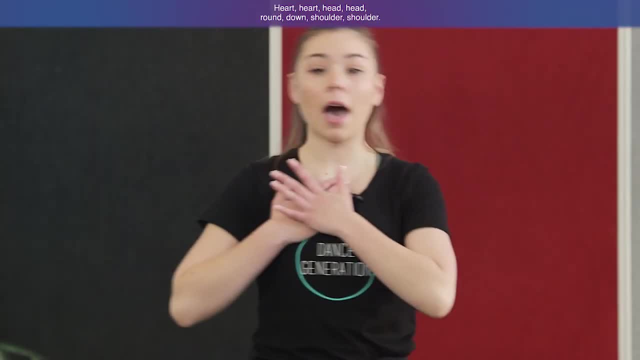 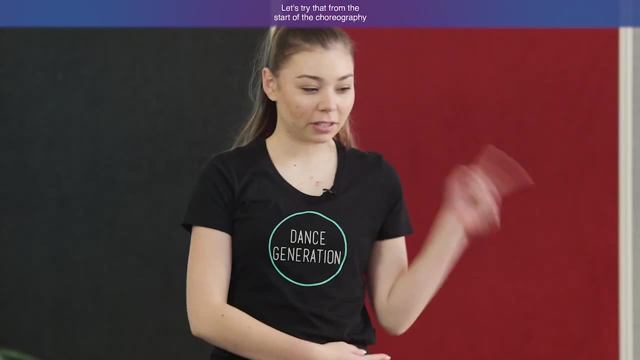 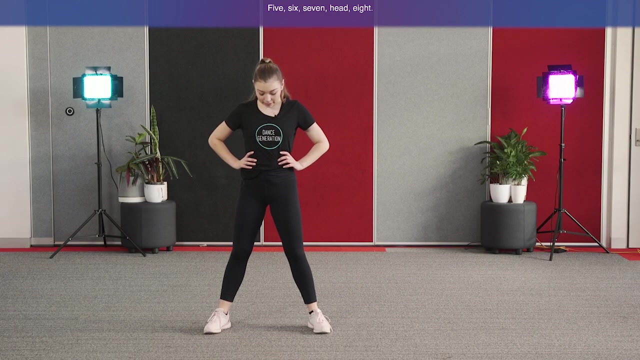 point shimmy, point heart, heart, head, head round down shoulder, shoulder. Let's try that from the start of the choreography to there, without any music. So we're feet apart, head down five, six, seven, head eight, We go. stamp, stamp, hip, hip, stamp, stamp, hip, hip. 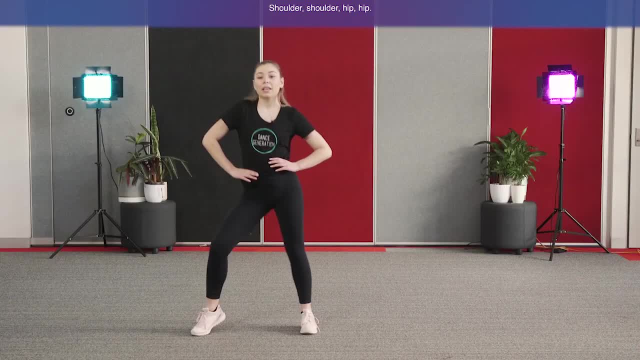 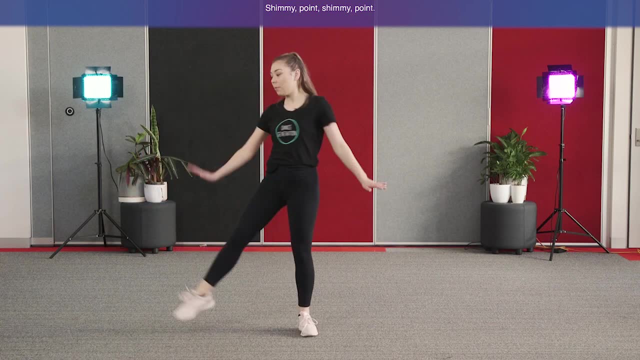 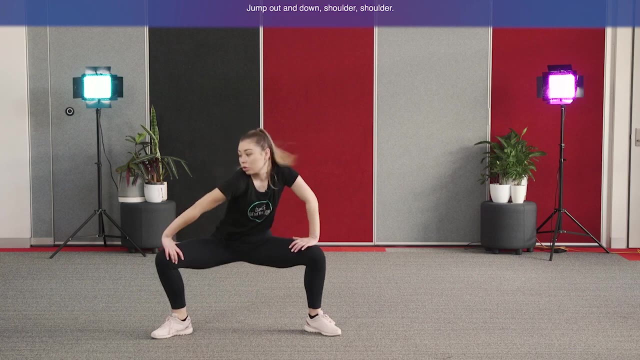 shoulder, shoulder, hip, hip, shoulder, shoulder, hip, hip. We jump it out down up shimmy point, shimmy point, heart, heart, head, head. jump out and down shoulder, shoulder, Good. One more time then to music Jump. 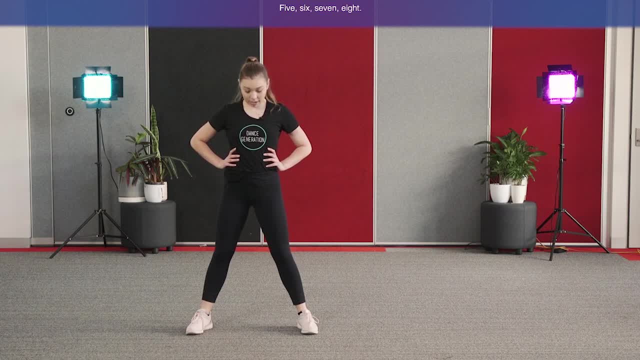 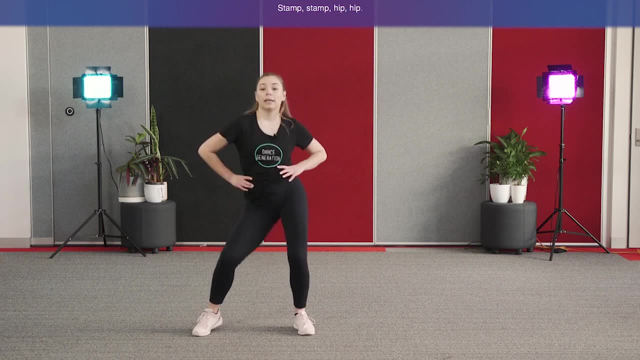 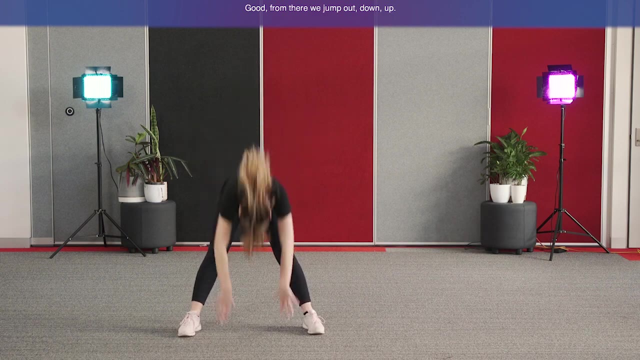 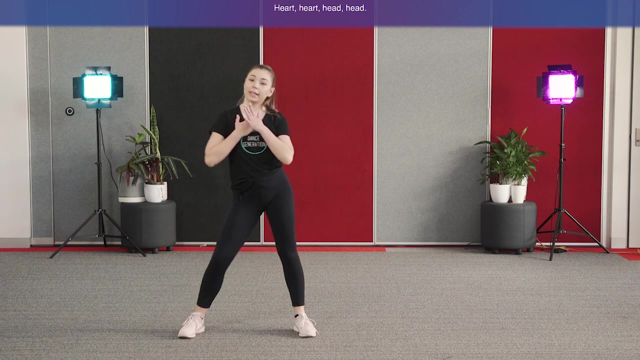 out five, six, seven, eight, We go. stamp stamp hit hit, stamp stamp hit hit shoulder, shoulder, hip, hip, hip, hip, hip good, From there we jump out down up shimmy point, shimmy point, heart heart. 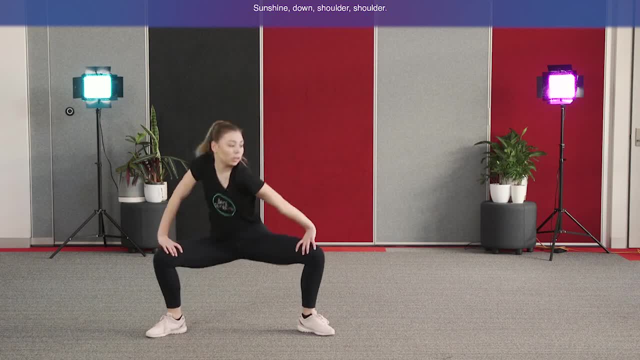 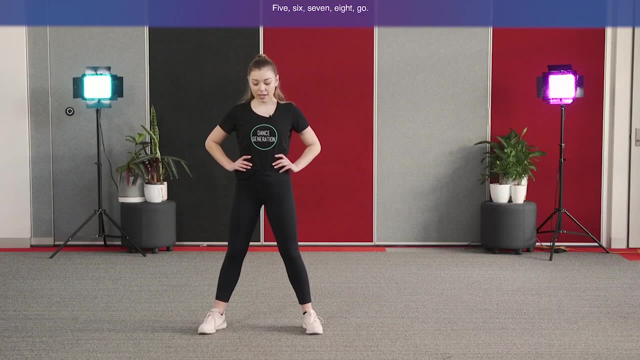 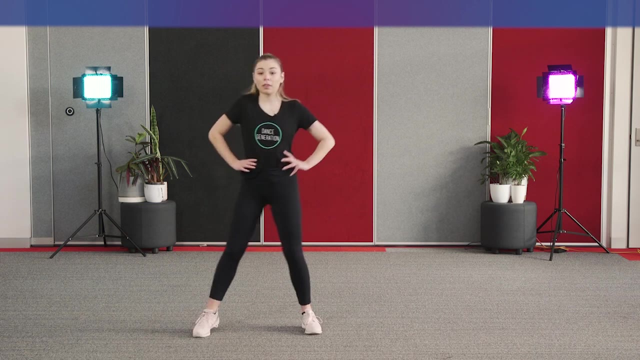 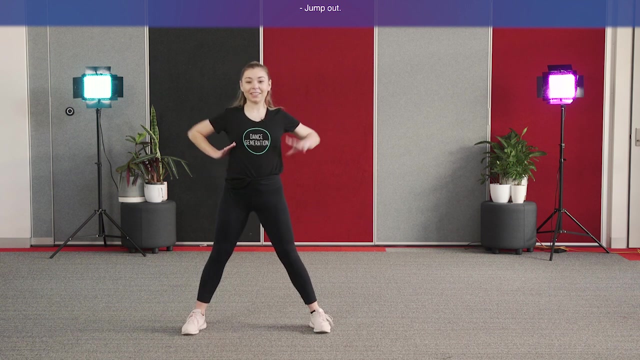 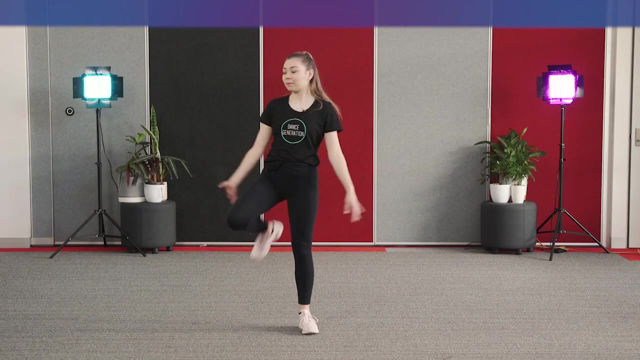 head, head, sunshine down shoulder, shoulder. Alright, let's tie that to the music from the start. Five, six, seven, eight, good Jump out, good shimmy head head, jump up down shoulder. 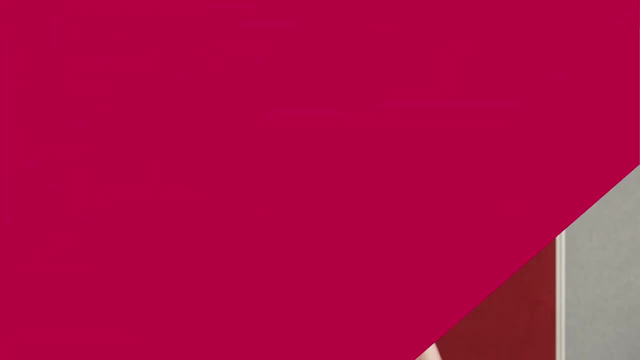 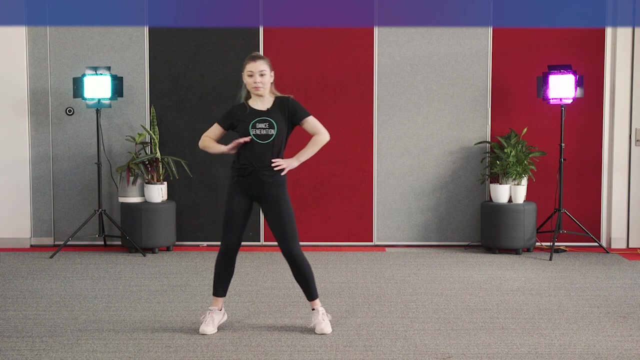 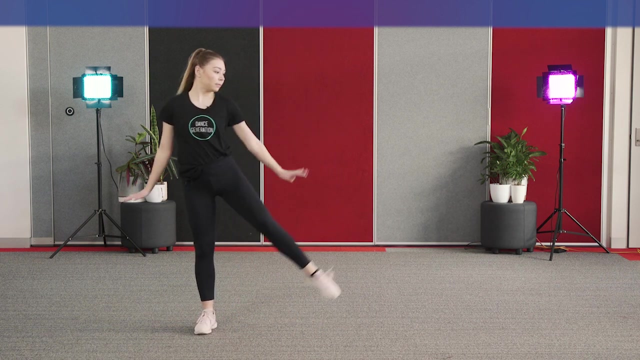 shoulder. good work, Let's try it one more time. Five, six, seven, eight, good, Jump out up, we go shimmy head head down. heart, heart, heart, heart, heart, heart, heart. 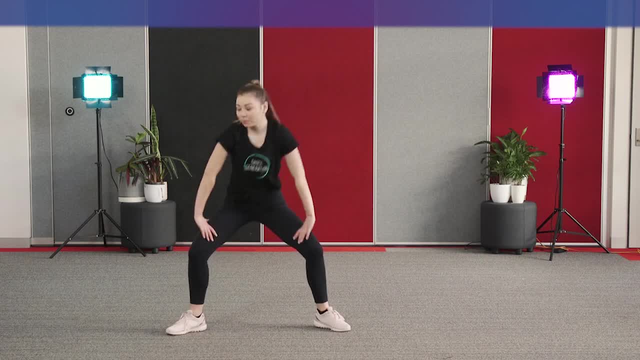 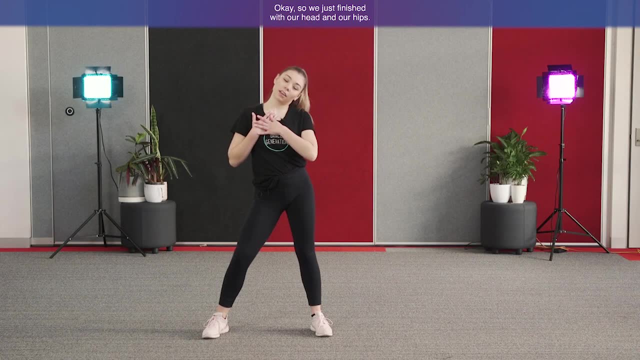 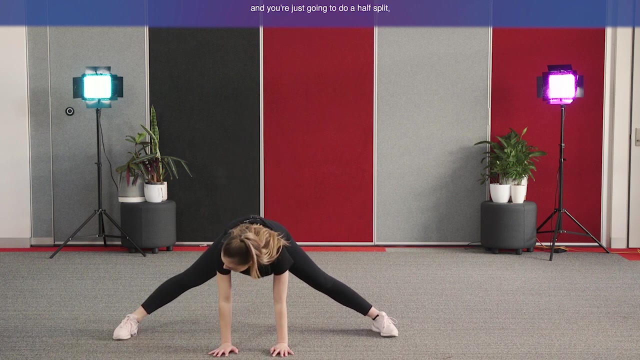 and shoulders. Good, Let's move on to the rest of the choreography. Okay, so we just finished. with our head and our hips, We jump around down shoulder shoulder, From here you're going to reach to the floor and you're just going to do a half split, or a full split, if you can. 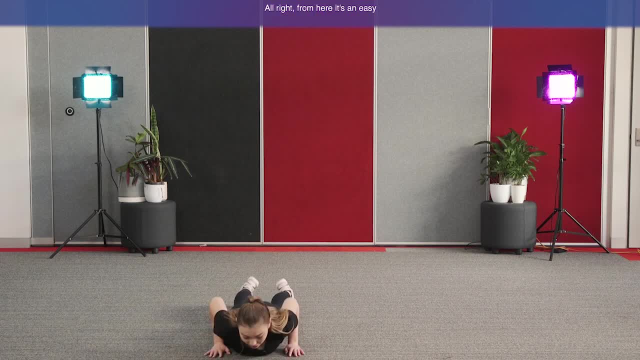 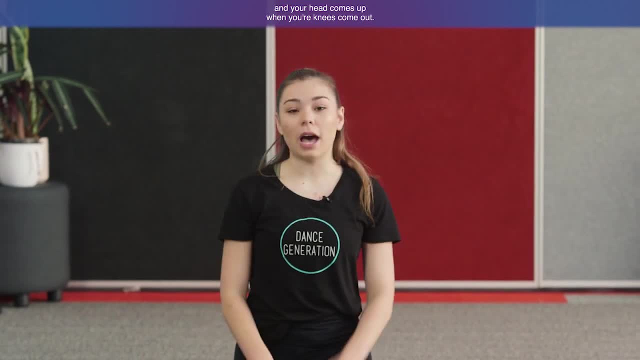 half a split, one more state. So we're not going to rest with our head on our knees All the way to our knees, So we're just going to jamais capture our knees. our head is down and your head comes up when your knees come out. So you go in out. good, You do two circles. 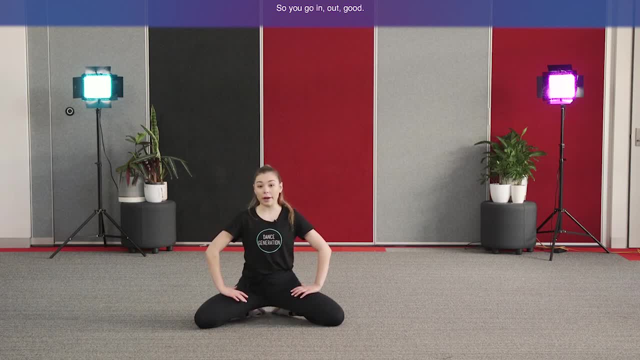 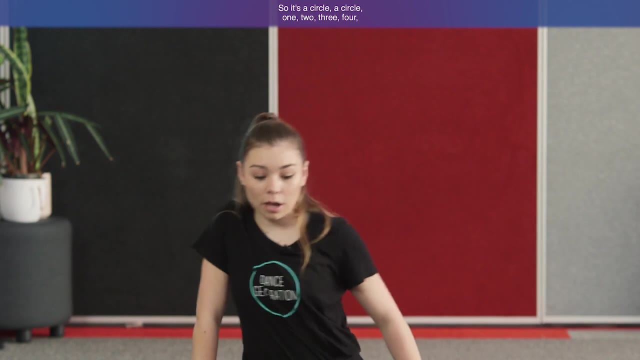 two, and then you do one, two, three, four. Side to side shoulder rib, three, four. yeah, So it's a circle. a circle: one, two, three, four. Hands on the floor, jump in. 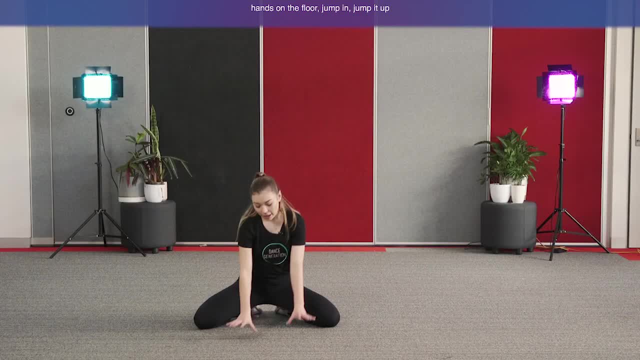 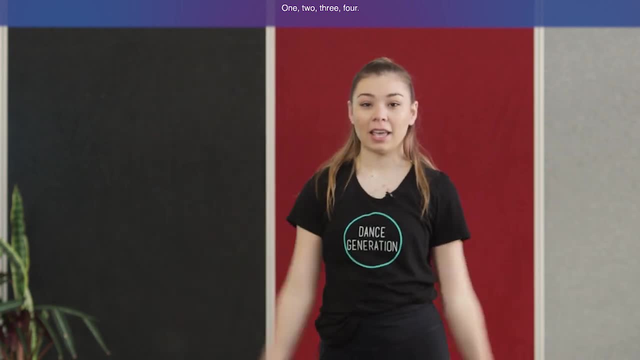 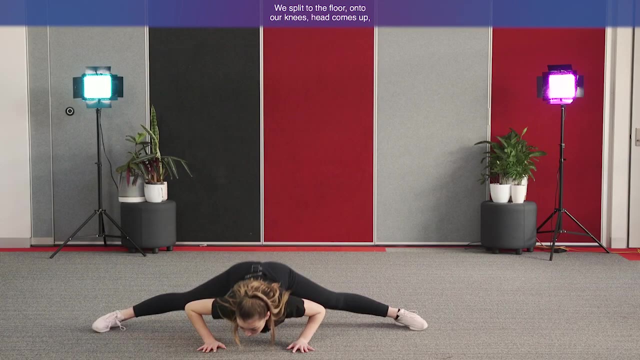 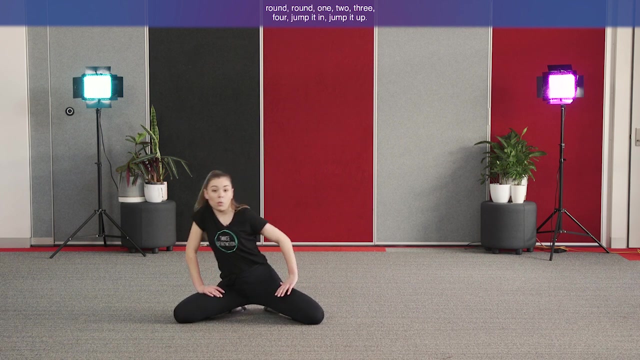 jump it up and we've got shoulders down خيابةatan, the knees come up, vibrating legs, legs, legs. strong arms. one, two, three, four, yes, so we've just done. big sunshine down shoulder shoulder. we split to the floor on. Chinese head comes up round, round one. 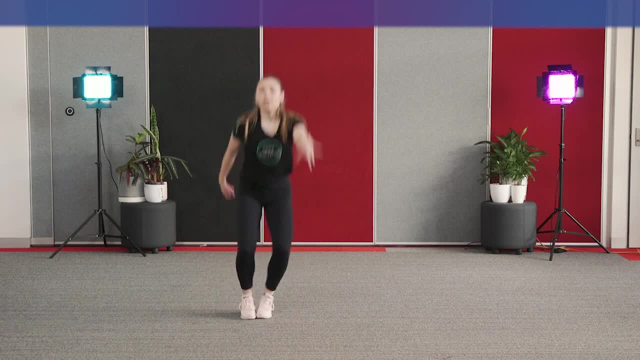 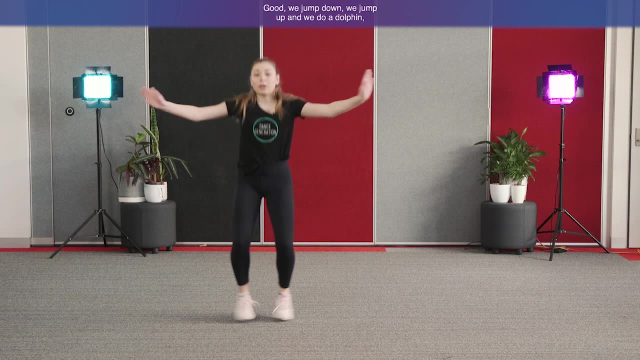 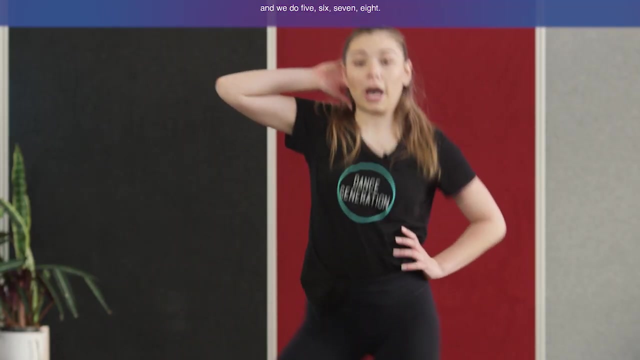 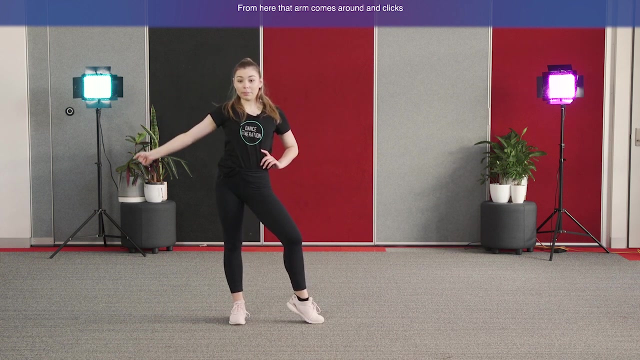 two, three, four. jump it in. jump it up. go one, two, three, four. good, jump down, we jump up. I'm gonna do dolphin body roll. hold it to here. I do five, six, seven, eight. from here that arm comes around and clips, clicks. go one, two, three, four, yes so. 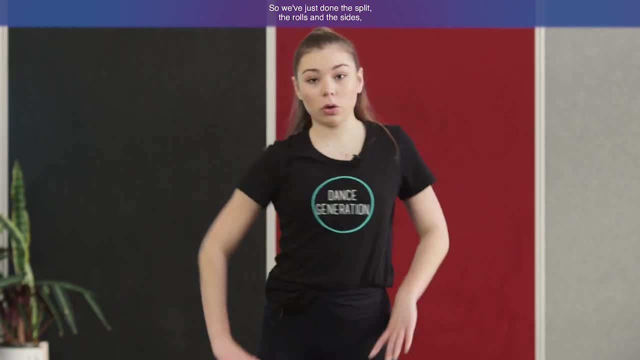 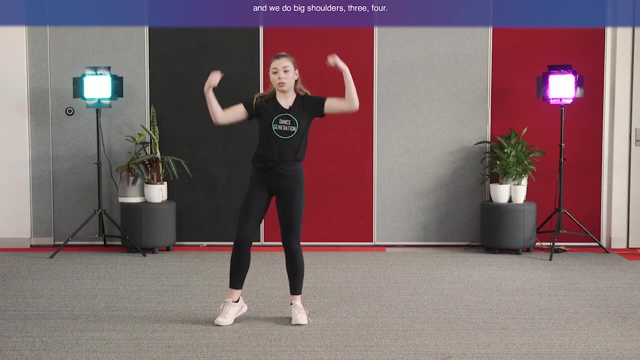 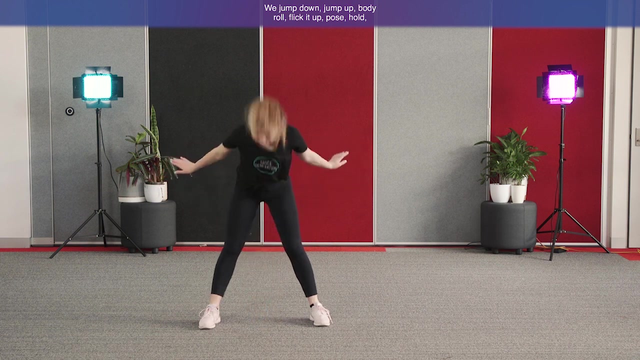 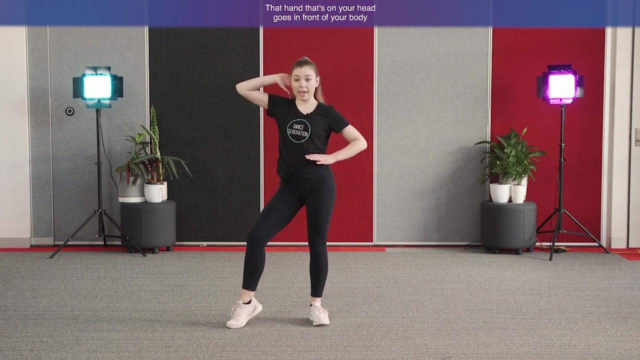 we've just done the split, the rolls and the sides. one, two, three, four: we jump together, jump up and we do big shoulders. three, four: we jump down, jump up, body roll, flick it up, pose, hold. one, two, three, for that hand that's on your head, goes in front of your body and you go five. 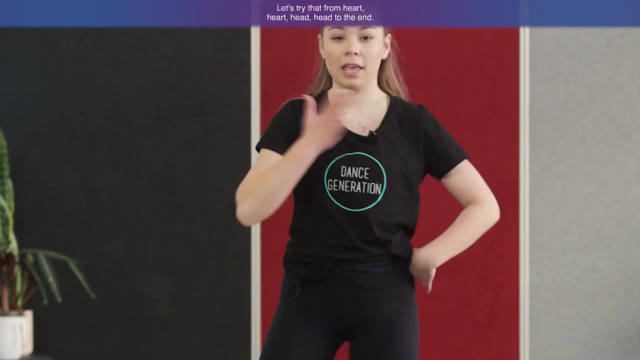 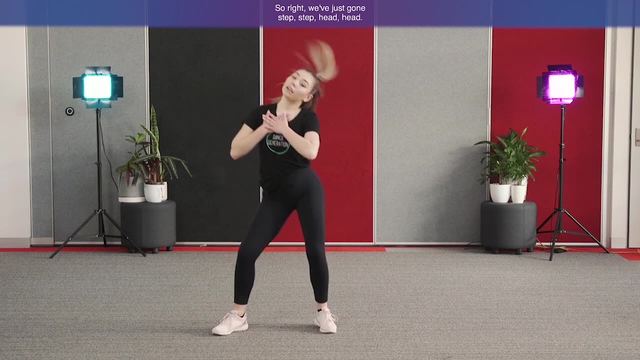 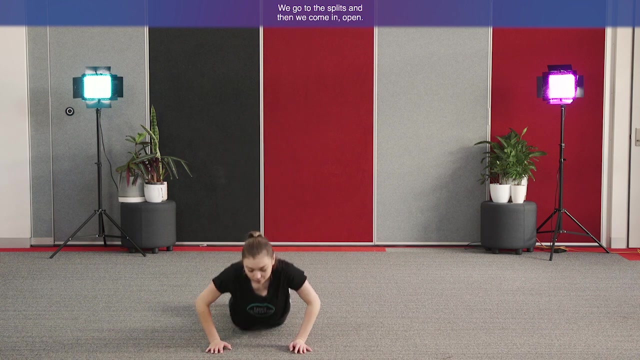 six, seven, eight. let's try that from hot, hot head, head to the end. so we've just gone step, step here, head we jump up, down shoulder, shoulder, we go to the splits and then we come in. I plan we go round round: one, two, three, four, jump in, jump up five, six, seven, eight. 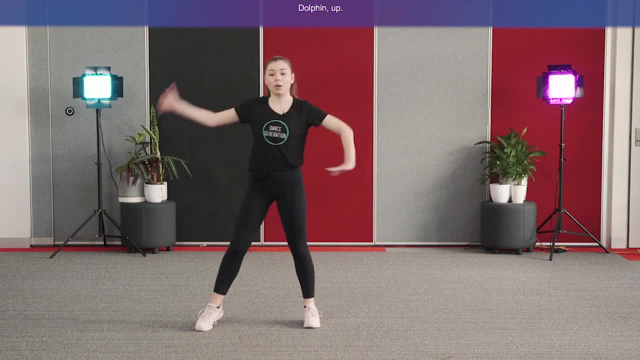 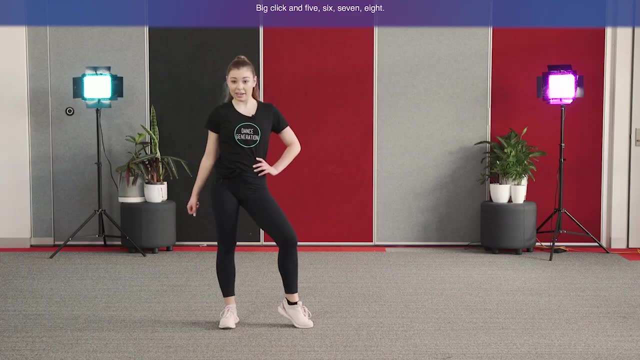 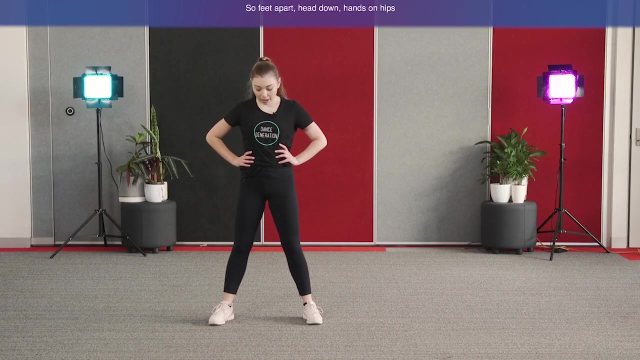 ah, dolphin, up, hold one, two, three, four, big click, and five, six, seven, eight. let's try that from the start. let's try that from the start, without any music, from start to finish. so feet apart, head down, hands on hips, and your head comes up on the count eight, let's go. five, six, seven, eight, we. 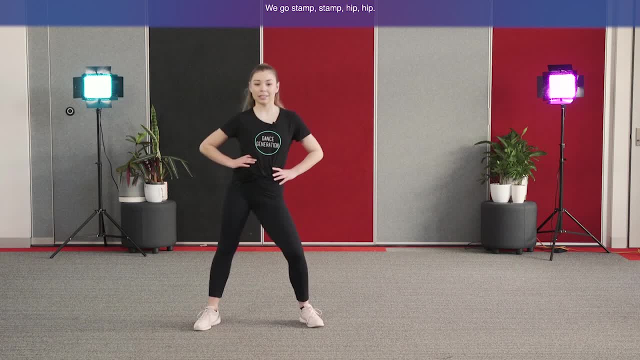 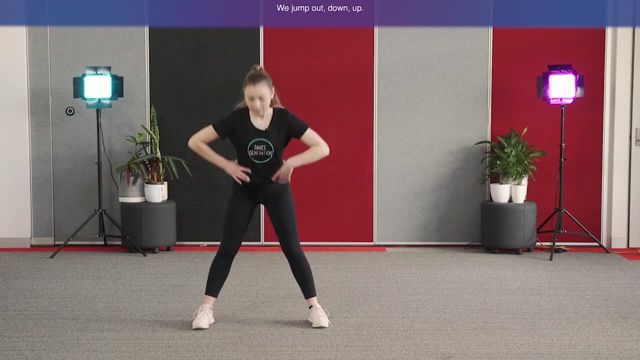 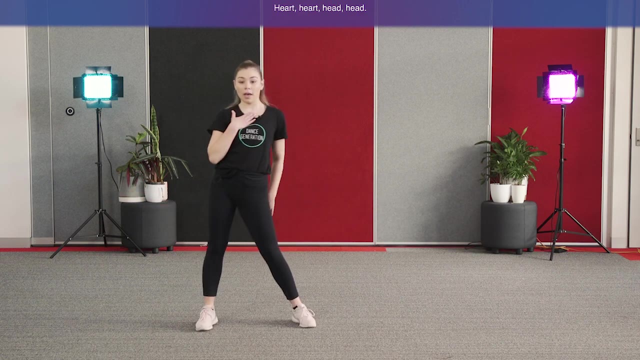 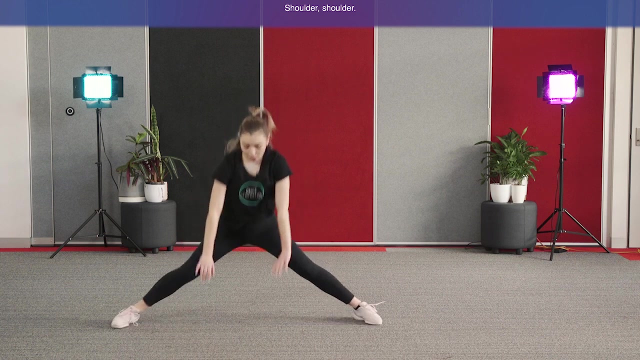 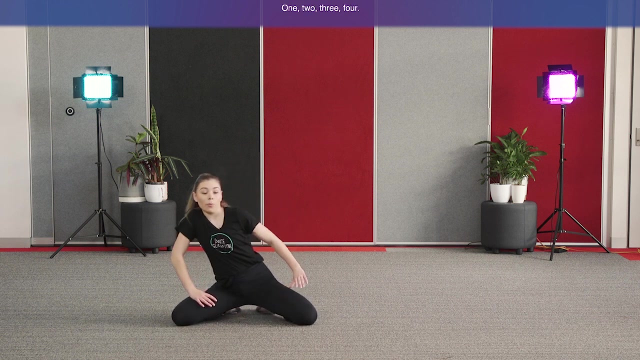 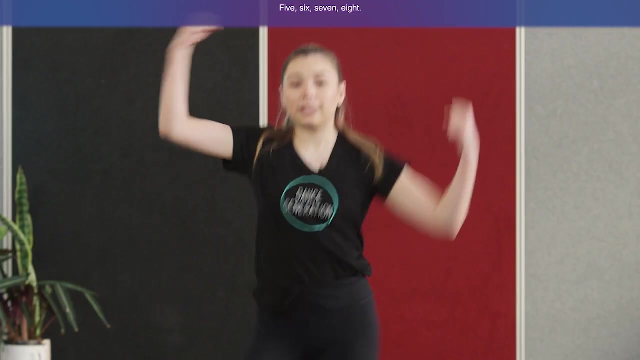 go, step, step, hit, hit, step, step, hit, hit shoulder, shoulder. jump out down up you shimmy point, shimmy point, heart, heart, head, head. big. jump down shoulder shoulder to the floor in up round round. one, two, three, four, jump in up- this is a fast one. jump in and up. five, six, seven, eight. jump in, jump out, dolphin. 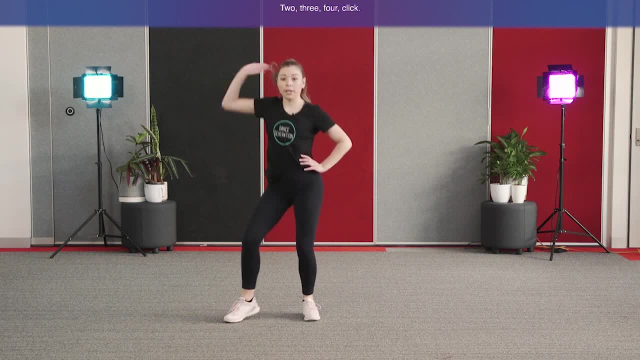 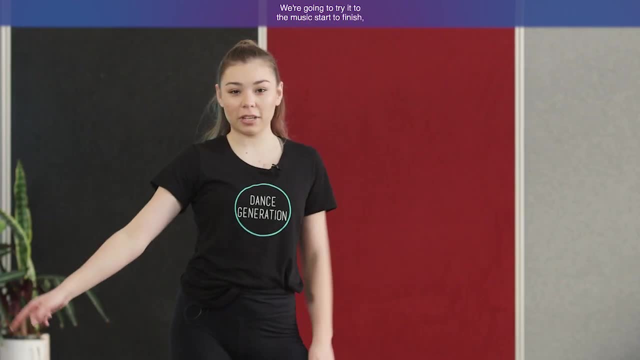 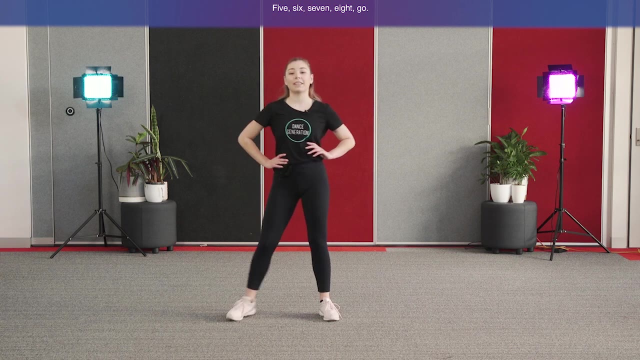 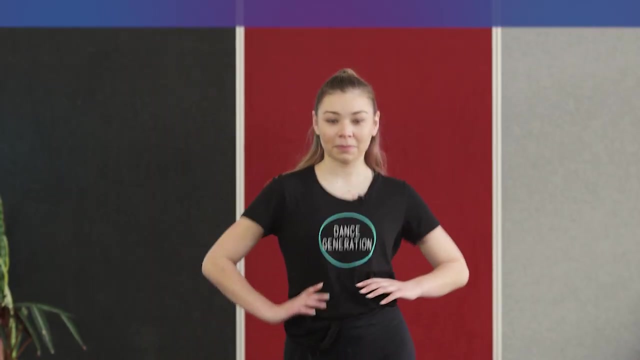 dolphin up. hold two, three, four, click five, six, seven, eight. good job everyone, we're going to try it to the music. start to finish a few times: five, six, seven, eight, take it. i should have said it before trying to hide it, fake it, rip. i can't pretend anymore.